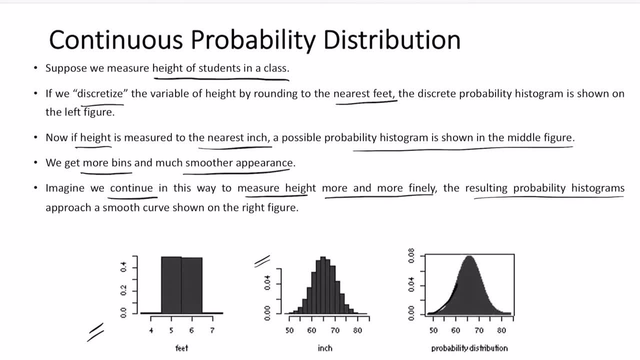 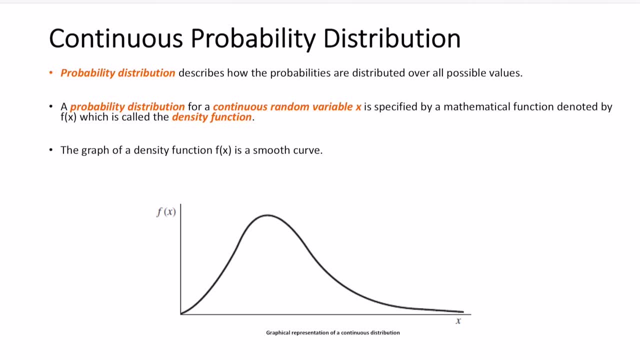 so the resulting probability histogram so appears to be a smooth curve. so because of this reason we call these distributions continuous probability distribution. So a probability distribution basically describes how probabilities are distributed over all positive possible values of x. Now a probability distribution for a continuous random variable x is specified by a mathematical function denoted by f of x, and this f of x is: 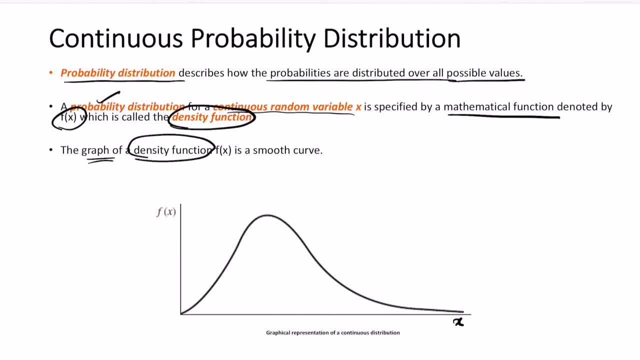 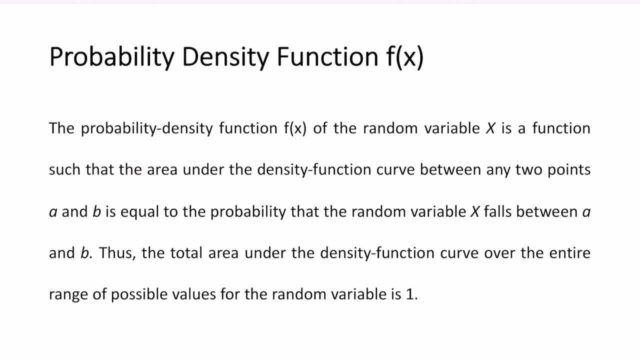 called as the density function. So the density function, the graph of the density function is generally has to be a smooth curve for it to be a continuous probability distribution. So to represent this continuous probability distribution we use probability density function. So if you remember from discrete normal distributions we call it as probability. 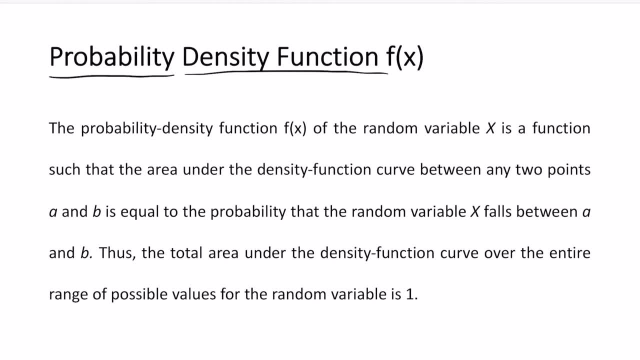 mass function because those are specific values, but here we call this probability density functions because these values have a density function curve between two points. a and b is equal to the probability that falls between a and b. So the total area under the density function curve over the entire range of possible values of the random variable is always equal to 1.. 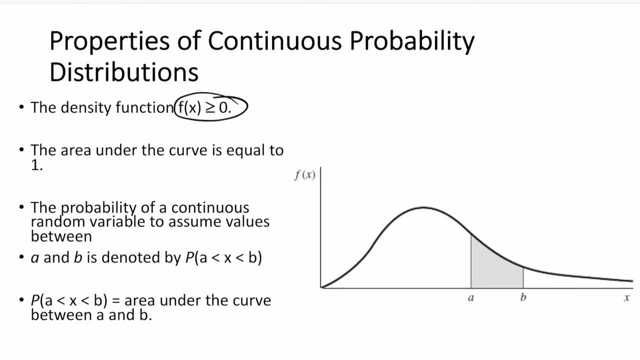 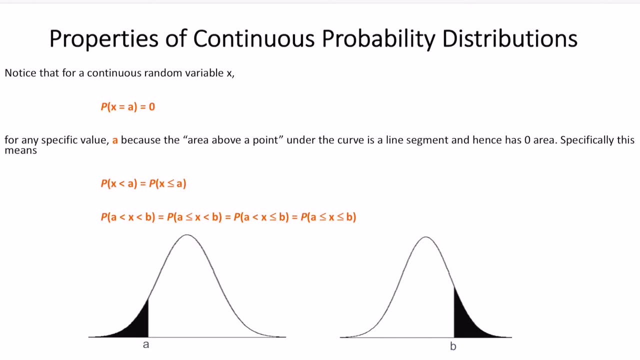 So these are the two main properties. the density function is always greater than or equal to 0 and the total area is always equal to 1, and the probability between two points a and b is the area between those two points a and b. So this is how we can calculate the values. 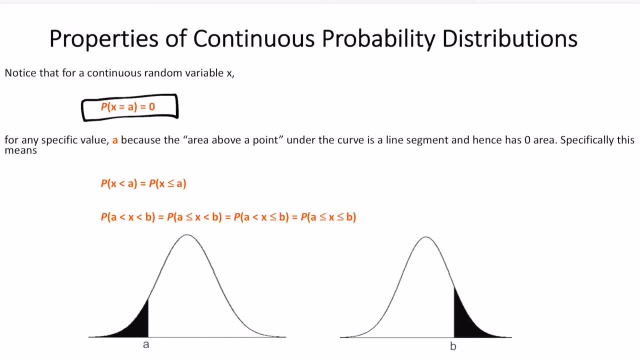 Now what are the other things? probability of one single specific value is always nearly equal to 0, because you cannot have a single value when you have a continuous probability distribution. So for any specific value of a, the area above the area will always be equal to 0.. Now one way to do this, most common way. 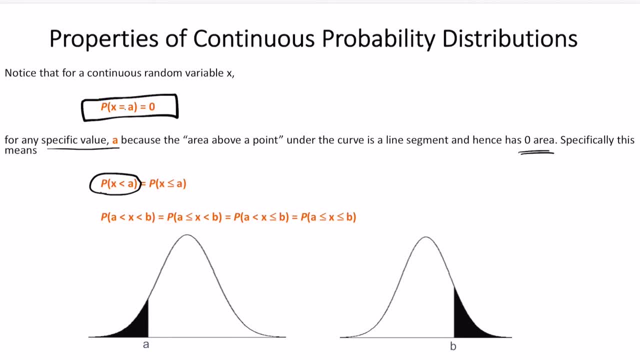 is to take less than. but remember that, because equal to is a. 0 less than a is the same as x, less than or equal to a. In the same way, p of a less than x, less than b is the same as a less than or equal to b, x less than or equal to less than b, and all these. 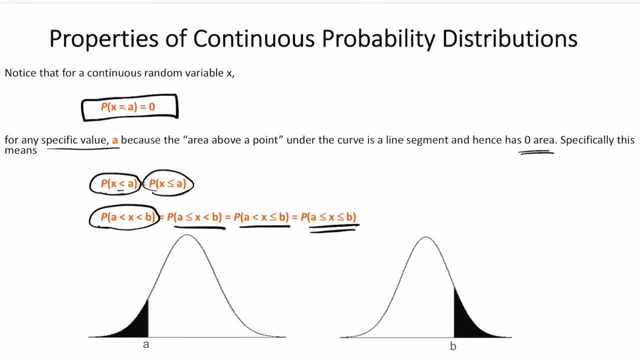 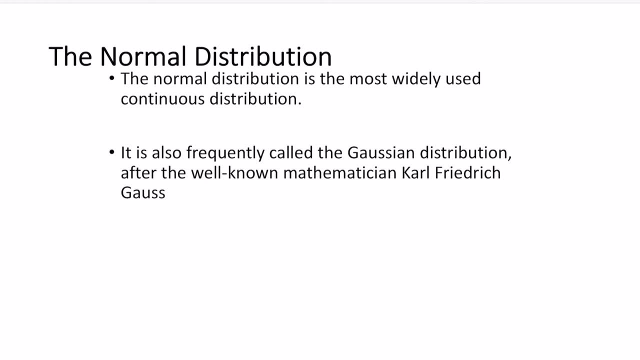 versions, because at a specific value there is no probability, So you can write it in different formats. Now, one of the common forms of probably continuous probability distributions that is more commonly used than any other is the normal distribution, So this is the most widely used continuous probability distributions. 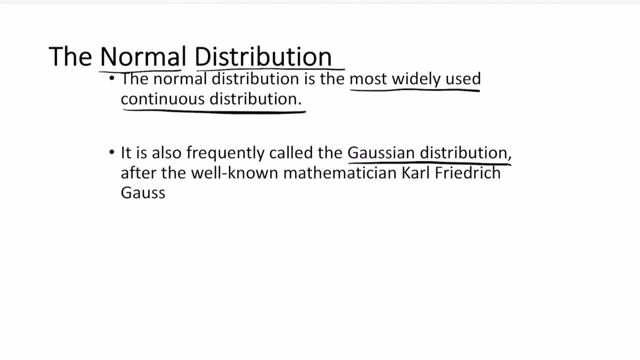 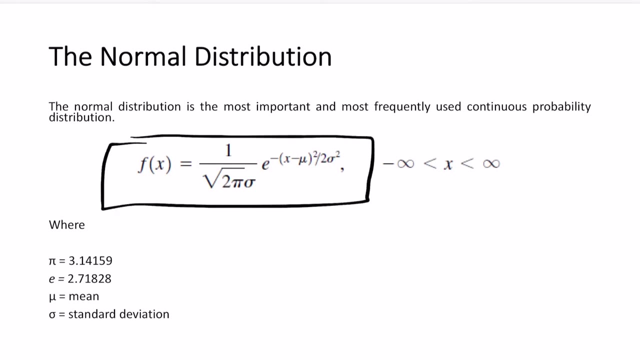 The other name is Gaussian distribution, Known because of the well-known mathematician Carl Friedrich Gauss. So if you see Gaussian distribution or normal distribution, both mean the same. Now, what is the normal distribution? so this is the equation that represents the probability density or the density function for the normal. 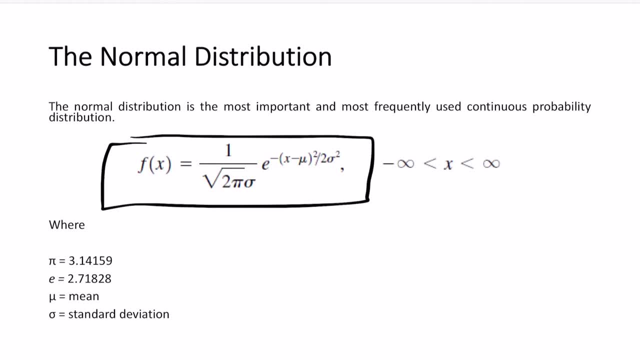 distribution equation. So 1 by 2 under root 2 pi and times Sigma into e, to the power minus of x, minus mu, squared by two Sigma squared, So again pi is 3.14.. e is 2.71, mu represents the mean and sigma represents the standard deviation, because 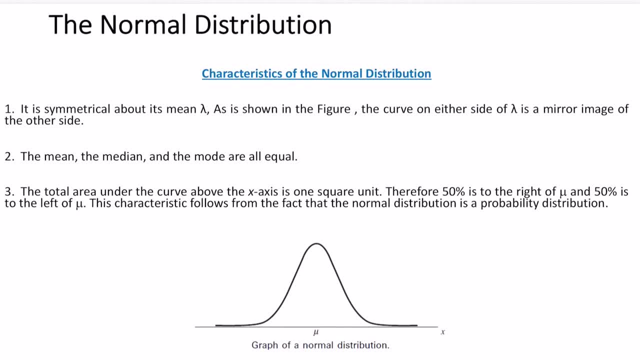 this formula is complex. what we try to do is we try to standardize this. so before we try to understand standardization, let us discuss the characteristics of a normal distribution. so the first characteristic is that it is symmetrical about its mean. so if you take the mean, it splits. 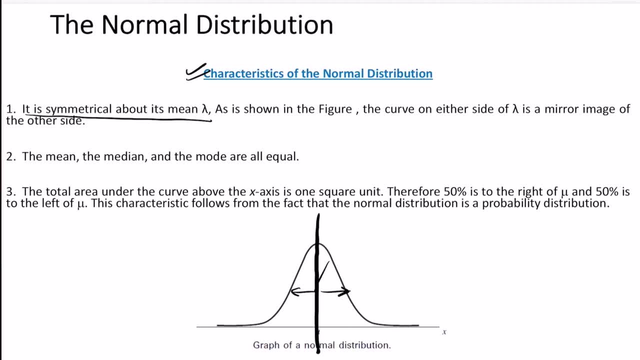 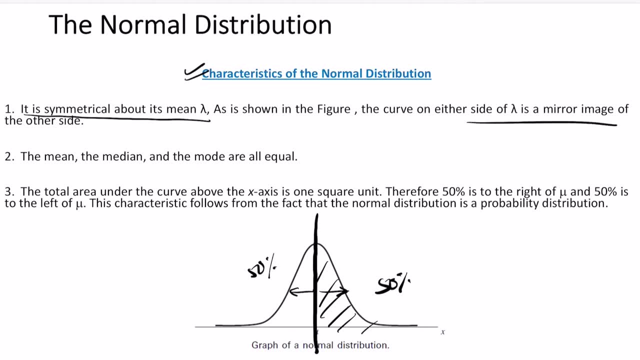 the two parts, so two. it splits it into two equal parts, so this becomes 50 percent and this becomes 50 percent, and the curve on either side is a mirror image of the other. so both are mirror images of each other and the mean, median and mode are all equal. so this is the point where 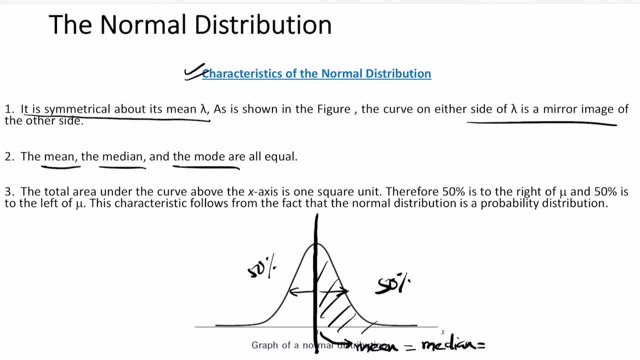 mean is equal to median, is equal to mode. next, the total area under the curve above the x-axis is one square unit, so the total area under the curve, so sigma p of x equal to x or sigma f of x. so we do not use sigma f of x. 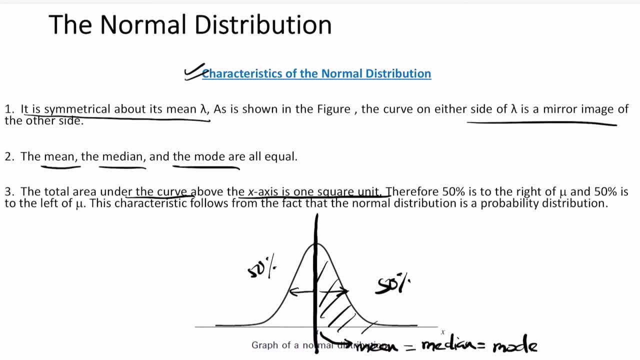 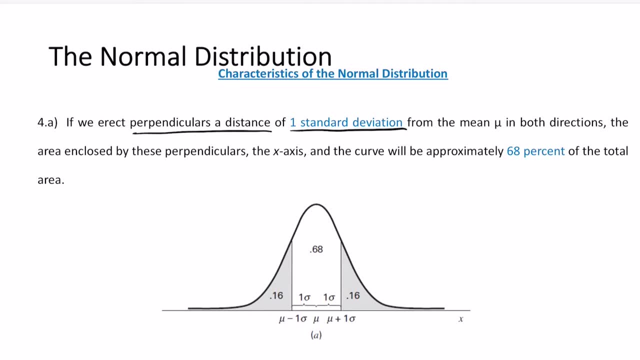 sigma f of x, but the total area is always equal to one next four if you erect two perpendiculars at a distance of one standard deviation. so, for example, if you take from mu, if you take one standard deviation to the left and one standard deviation to the right, which is between mu minus sigma and mu plus, 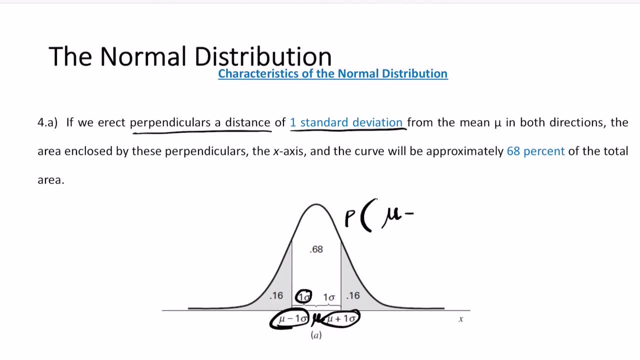 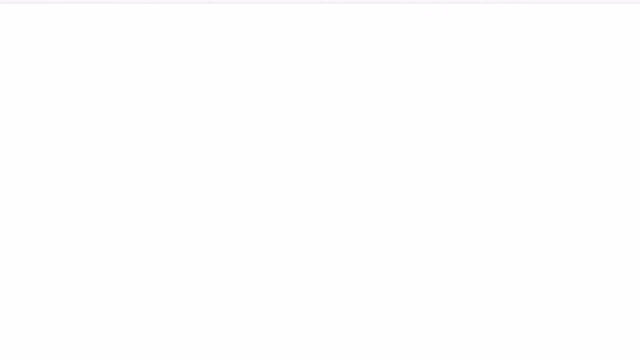 sigma. so the probability of mu minus sigma less than x, less than mu plus sigma, is 68 percent or 0.68. so this is the property for any value of mu and sigma, provided that the mu and sigma abide by a normal distribution. now the same rule also applies for two sigma, and so p of mu. 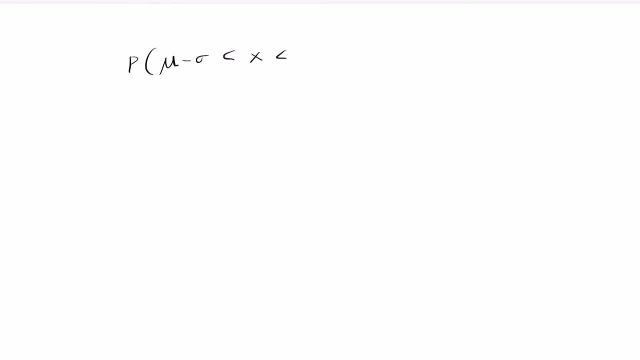 minus sigma, less than x, less than mu plus sigma, is equal to 0.68 or 68 percent. so p of what is 2 sigma, 2 times the normal distribution, 2 times the standard deviation, mu plus 2 sigma is going to be 0.955 percent. and p of mu minus 3 sigma, less than x, less than mu plus 3 sigma, is 0.997 or 99.7. 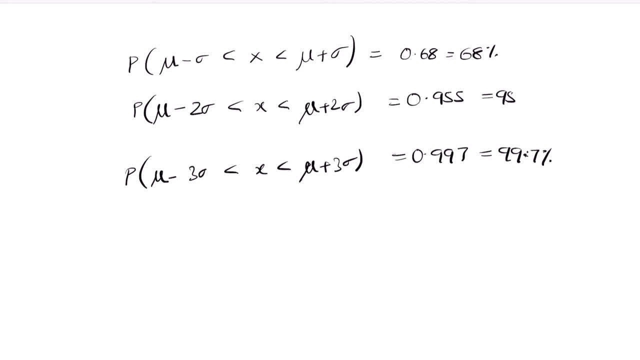 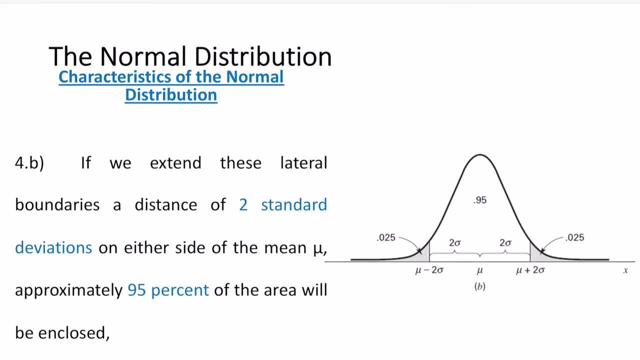 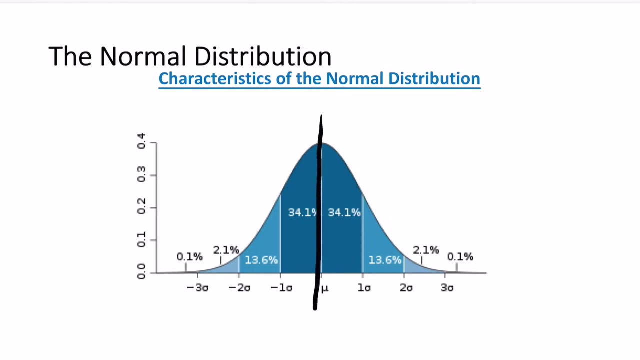 percent. I am sorry, this is 95.5 percent. So this is how we can, based on the standard deviation value. so these are the values. Now, if you split it equally- because it is symmetrical across this axis- 68 percent generally, 68.2 percent- can be split into 34.1 and 34.1 until. 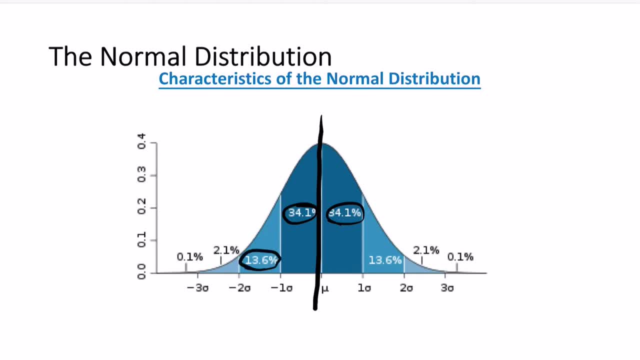 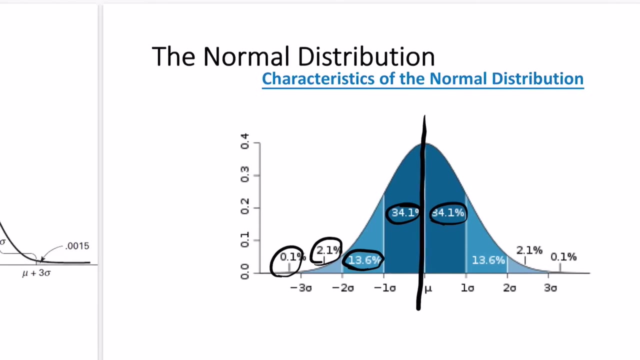 1 sigma. from between 1 sigma and 2 sigma, the value is 13.6 percent. between 2 and 3 sigma, that is 2.1 percent. anything above minus 3 sigma is 0.1 percent. so these are the values that you do, you can remember on on your hand. so between mu plus. 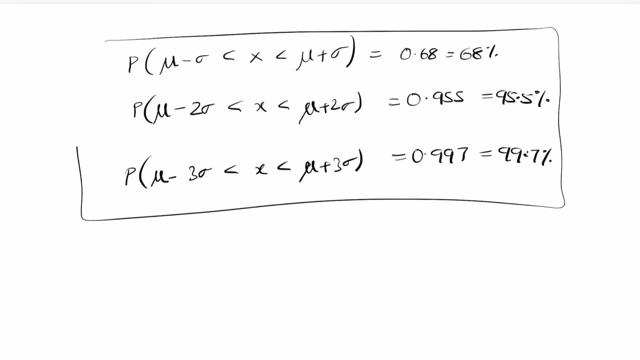 so this is the main part that you have to remember by heart, because most usmle problems. if they give you a value like this, they would generally mention it based on the values of mu and sigma, so it makes it easier to write down these values. next last characteristic is the normal distribution. 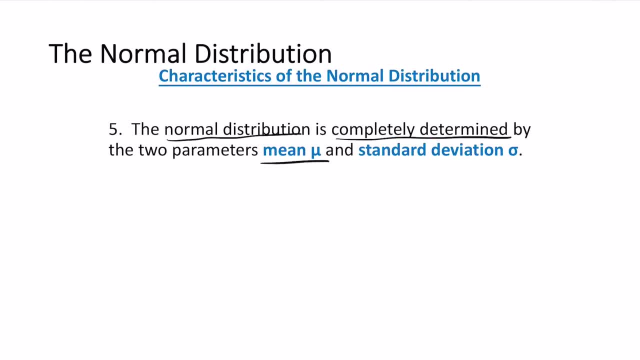 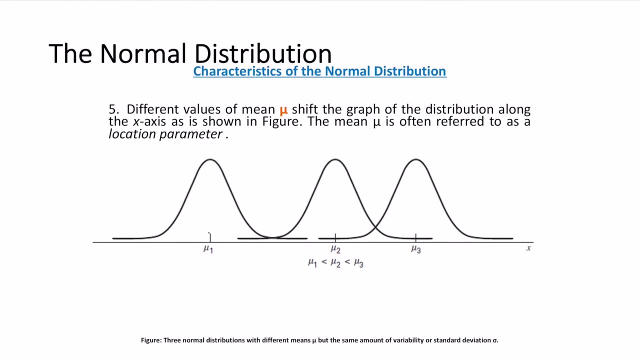 is completely determined by the two parameters mean and standard deviation. so for the entire, for the entirety of normal distribution, you just need to know the mean and the standard deviation. so with that two values, you can represent the entire normal distribution. now let's take a look at this diagram. so this value shows different means. so mu 1, mu 2 and mu 3. so because their 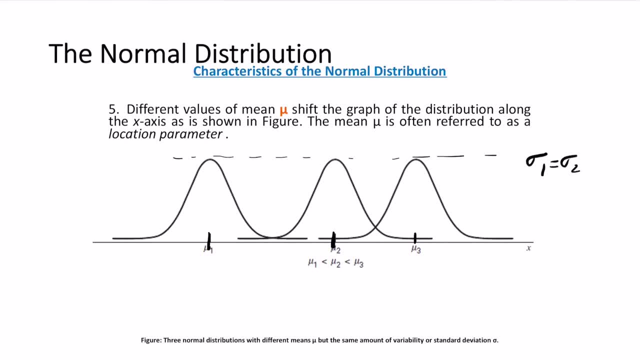 height is the same. they have the same significance. so sigma 1 is equal to sigma 2, equal to sigma 3.. So the height represents the sigma value and the center represents the mean. Now notice in this problem, all of them have the same mean. 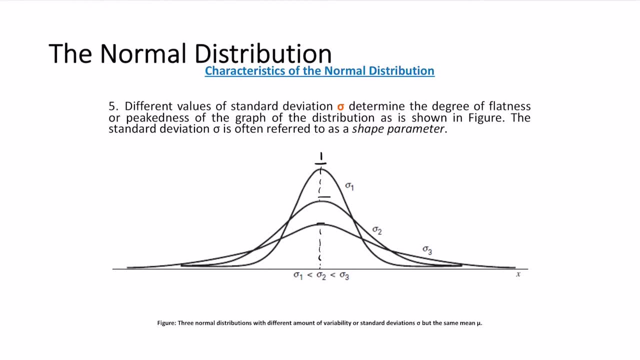 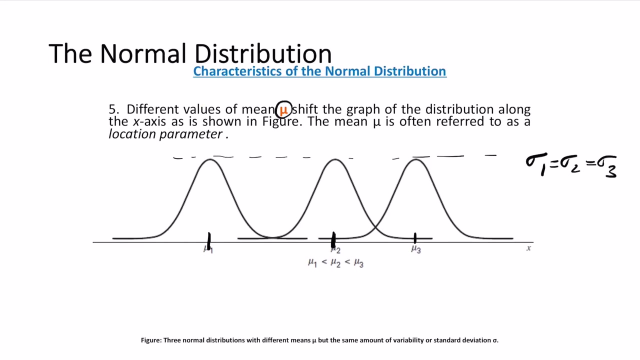 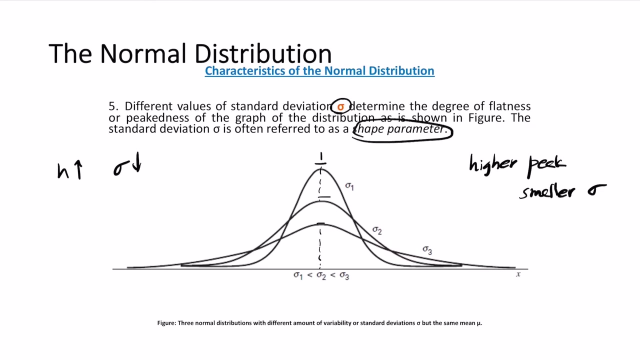 but notice the height. So the higher the peak, the smaller the sigma value. So as the height increases, the sigma value will decrease. So this is the relationship between height and the value. So here mu represents location parameter- where is it located- and sigma represents the shape parameter- how is it shaped? So these are the two variables that determine the 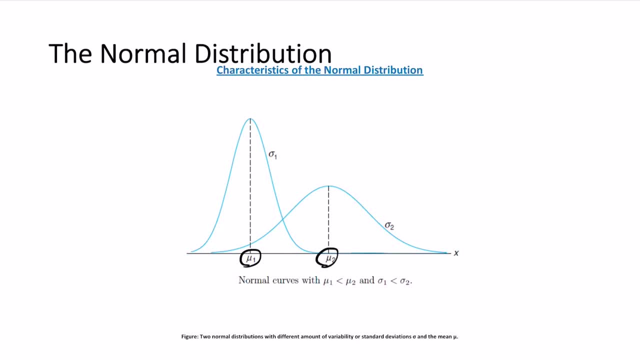 values. Now notice: here: mu 1 is here, mu 2 is here, So mu 1 is less than mu 2. here Sigma 1 is lot Higher and sigma 2 is smaller. So sigma 1 is less than sigma 2.. So this is how we compare. 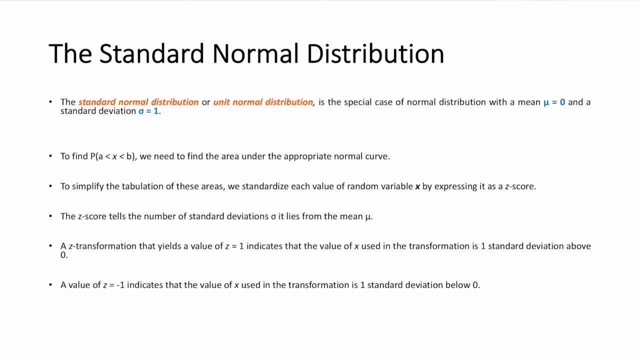 when you have two curves of normal distributions. Now let us take a look at the next one of how to standardize this normal distribution. So the way to standardize this is to take what is a standard normal distribution is a standard normal distribution is where the mean is 0 and the 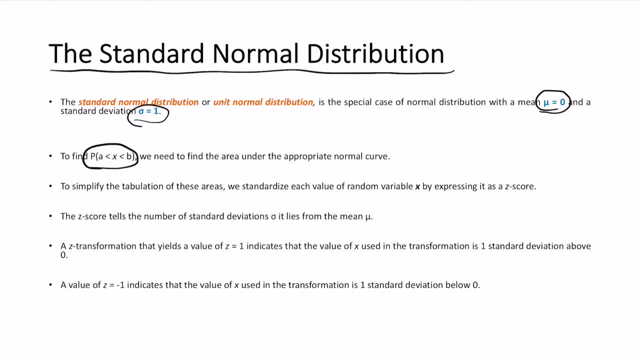 standard deviation is 1.. So to find any probability we basically find the area under the appropriate normal distribution curve. So for this what we generally do is we note down the z score. So the z score is the value that can tell you how much the 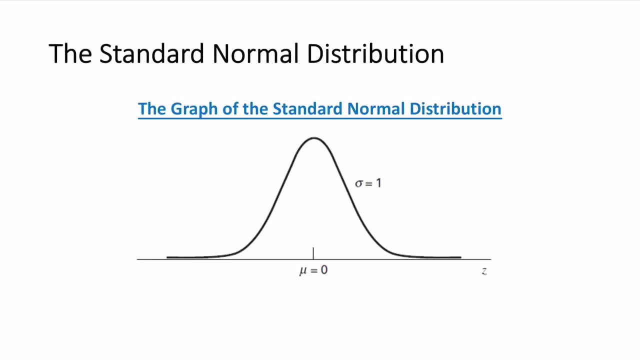 probability is. So when you take the z score. so the z score here represents the z distribution, is the value that represents the standard normal distribution. So how do you find this z score? is z value here is given by the formula. So this is the z score. So this is the z score. So this is. 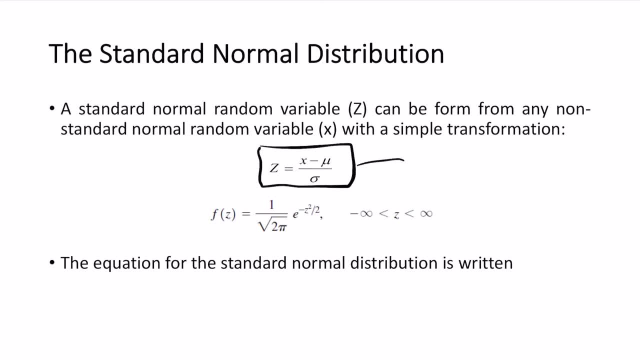 the formula x minus mu by sigma. This is the formula we use to convert a normal distribution into a standard normal distribution. So this is how we can convert a normal distribution into a standard normal distribution. Why do we need to convert it into a standard? So that we don't. 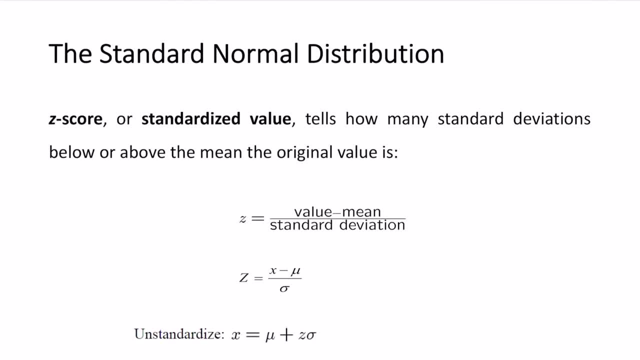 need to use the formula. this formula to calculate every single time. So the z score value is the standardized value is basically the z score is the standardized value, So we can calculate. the tells you how many standard deviations below or above the mean the original value is. so it. 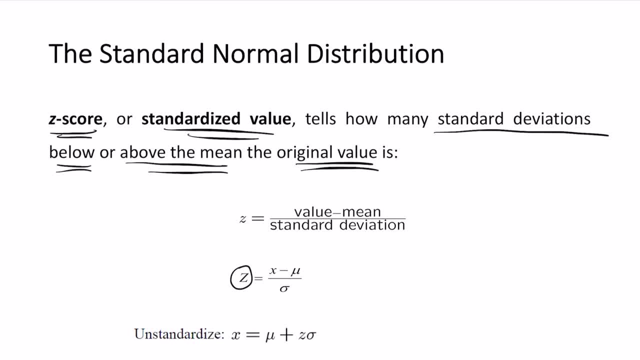 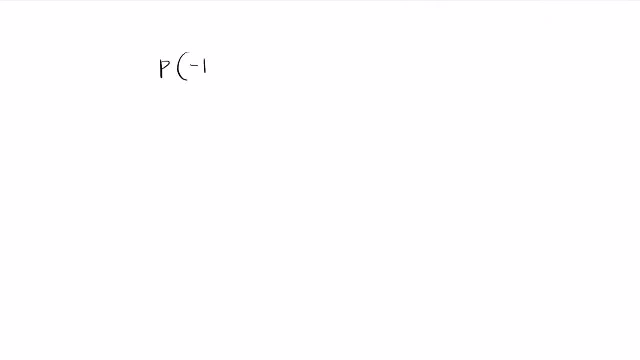 basically says whether the value is one standard deviation away or two standard deviations away. what does that mean? so if you take the probability of minus 1 less than z less than 1, that value is equal to 0.68. if the if you take the probability of negative 2 less than a, so negative 2 less than z. 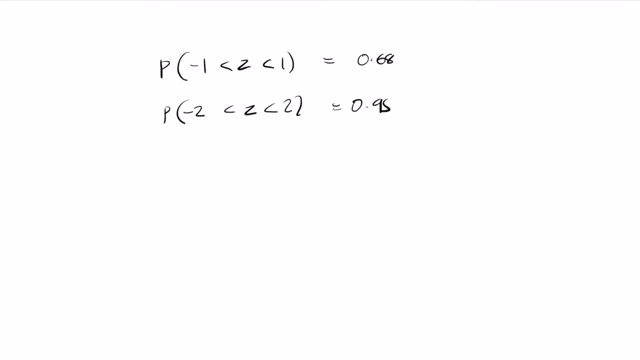 less than 2, that value is 0.955. and if you take the probability of negative 3 less than z, less than 3, that is 0.997. notice, notice: the values are exactly similar to what we did before because z score standardizing with the z score using a z score can help us find probabilities much. 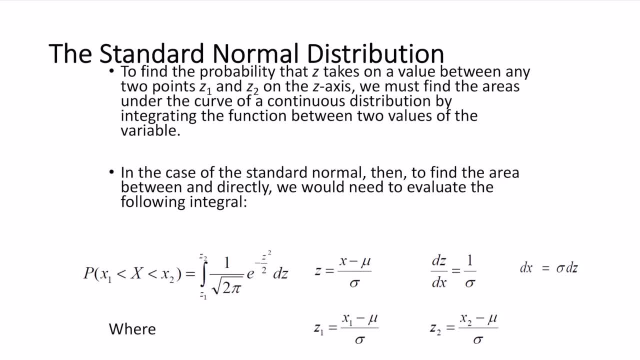 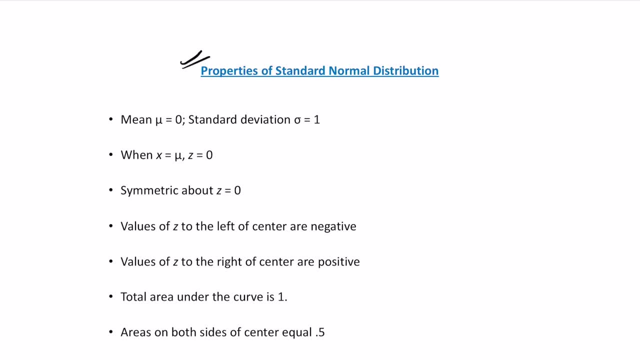 more easily rather than using the formula every single time. now let's try and understand how to find. so what are the properties of the standard normal distribution? so the first property is that the mean is 0 and the standard deviation is 1, and when x is b equal to mu, then the z value becomes 0, so which means that z equal to 0. 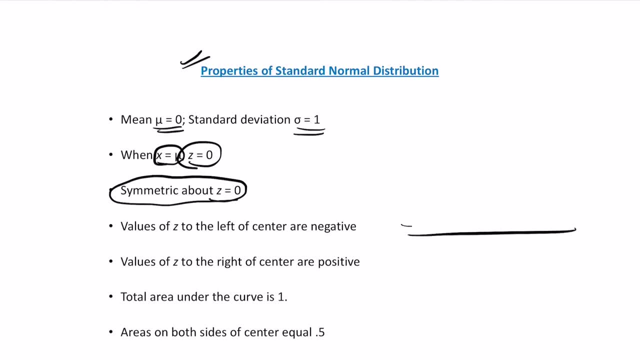 is the line that is symmetric. so if you take the distribution here, if you take the distribution here, so this is z equal to 0. any value to the less one is z is negative. left is negative, anything to the right is positive, but the total area under the curve is still 1 and each side represents 0.5. 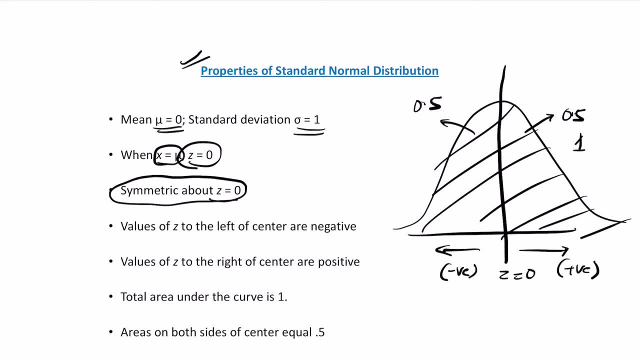 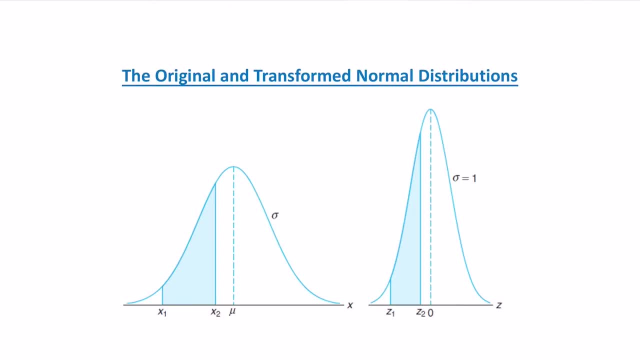 so each side represents 50 percent of the probability of the total function. now let's take some examples and let's try and see how do you convert a transformation from one side to the other and how do you convert a transformation from one side to the other. 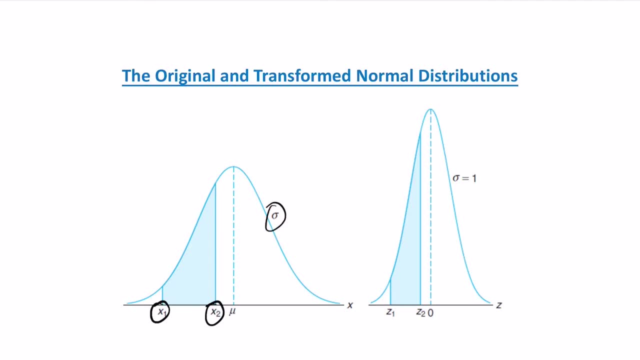 system into the other. So how do you convert a general distribution or general normal distribution into a standardized normal distribution is by using the z value. So what we do here is we take x1 value and we find out the z1 value, which will be equal to x1 minus mu by sigma. In the same way, 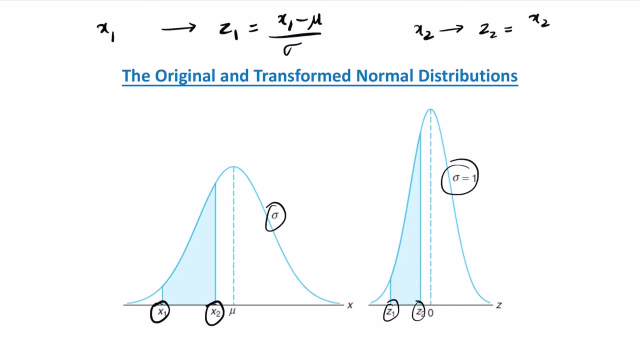 we take the x2 value and we find z2, which is going to be x2 minus mu by sigma. So by converting x1 to z1, we are basically converting it from normal to a standard normal distribution. So the the reason we do this is because standard normal distribution has a specific table. 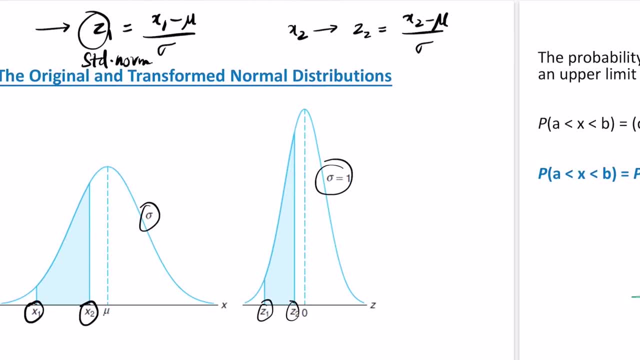 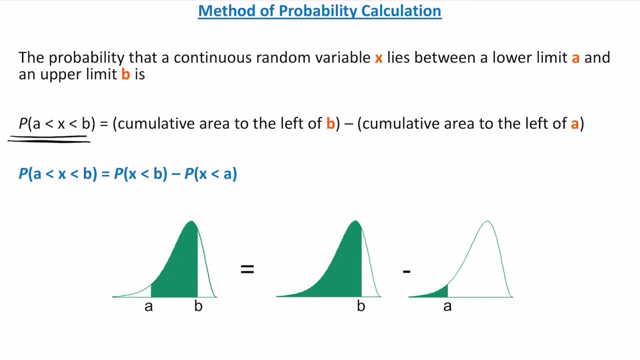 which can help us in finding out the probabilities much more easily. Now, how do you find when between in a graph? so how do you calculate from the table between a less than x, less than b? So the formula for that is p of x less than b. where 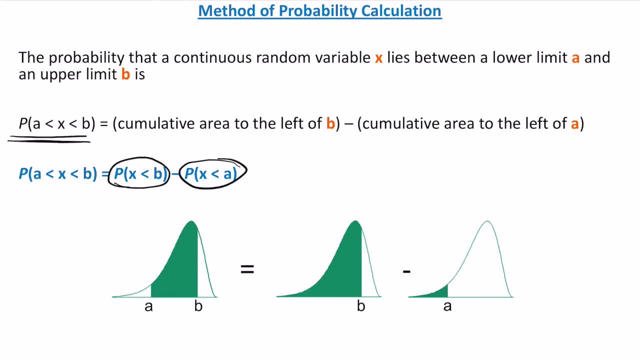 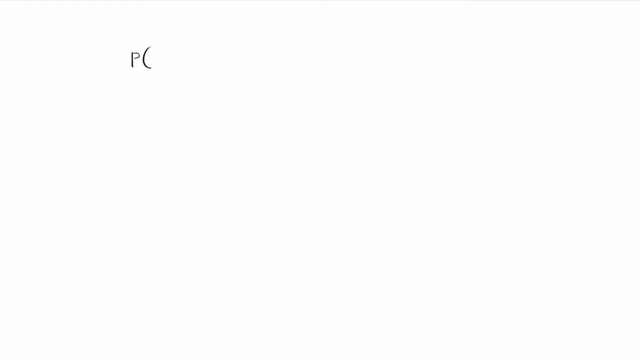 b is the greater one minus P of X less than A. So remember this formula because we are going to use this again and again. So let me write the set of formulas that we are going to use. So P of X less than A. 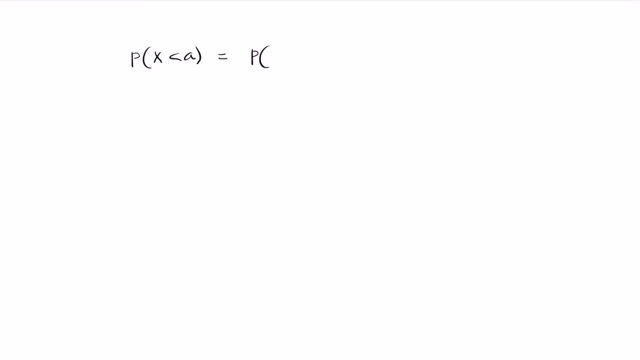 is directly found under P of Z less than some value of Z, Z1.. Let us call it Z1.. Next P of X. So, for example, P of X1 less than X, less than X2, is found as P of Z1 less than Z. 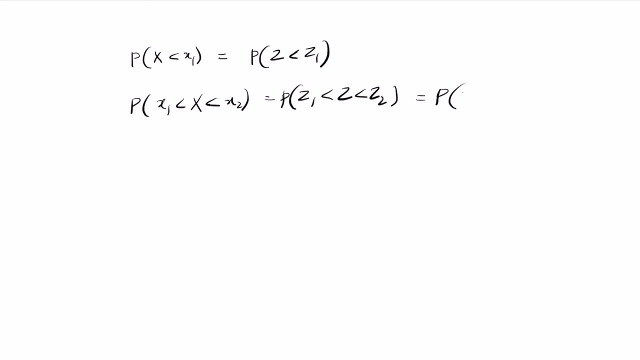 less than Z. This can be written as P of Z less than Z2 minus P of Z less than Z1.. So this is how we find it from the table. If you want to find greater than value, so X greater than X1,. 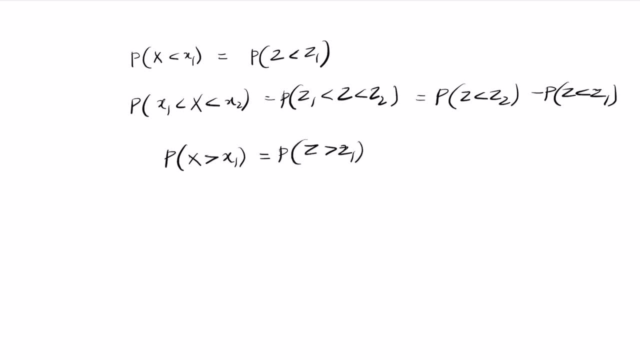 so we find it as P of Z greater than Z1.. So we cannot find this directly from the table. So what we do here is we write it as 1 minus P of Z less than Z1.. So these are the three set of. 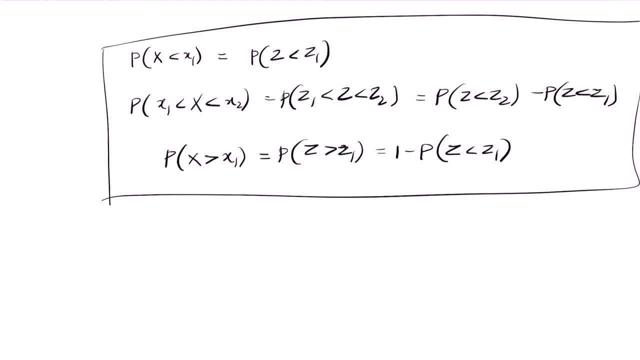 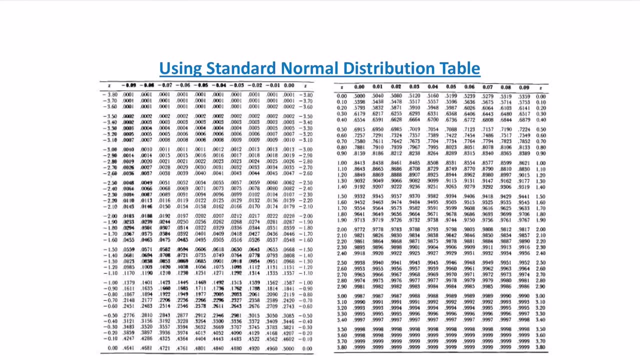 formulas that we are going to use in this chapter when we do the problem. So remember these set of formulas. Now, so to find the values of the probabilities, we use the standard distribution table, the normal distribution table. So this is the set of formulas that we are going to use in this chapter, So remember these set of 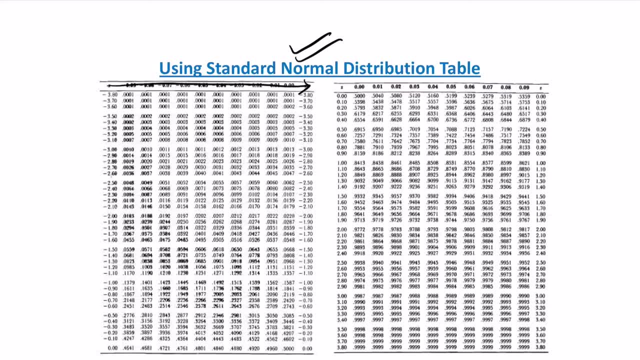 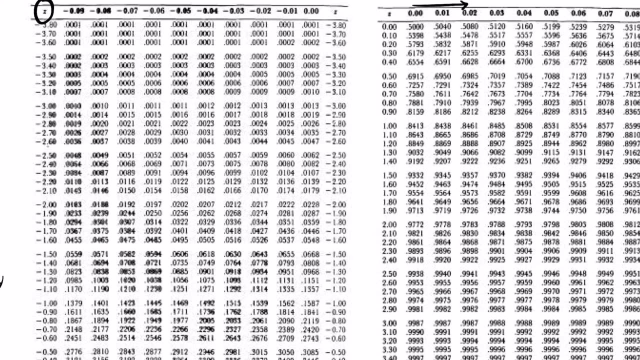 formulas. So this is the table. In this table, if you look at the first row, so the first row contains: so the first column contains the Z values. So these are all the Z values that you have. So these are all the Z values. And on the second, on the column part, we notice you have 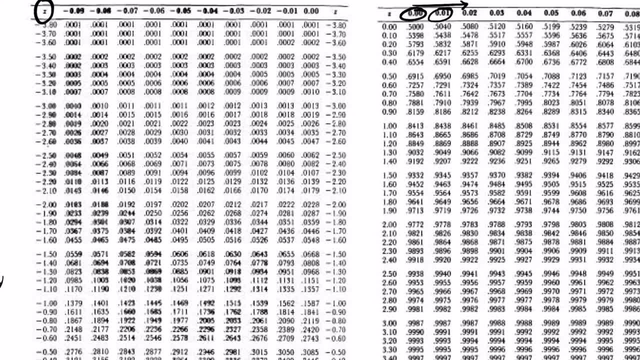 the decimal, the second decimal, which means that, for example, if I want to find minus 2.56, I am going to take minus 2.5.. In that I am going to find 0.06.. And that value is my answer. So this is the value for minus 2.56.. So you're basically finding until the. 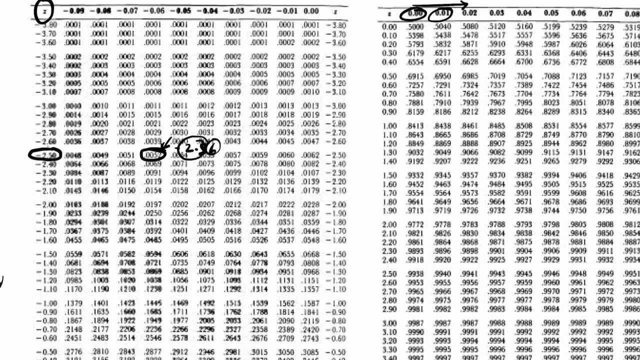 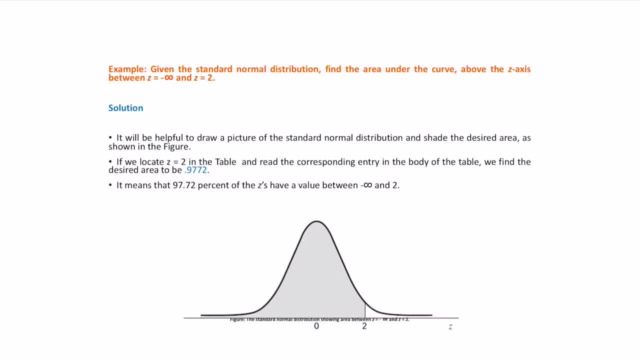 first decimal and the second decimal is the next row. So always take the values until two decimals so that it becomes easier to find the value. Now let's try and do a problem. So, given the standard normal distribution, find the area under the curve, above the Z axis, between Z. 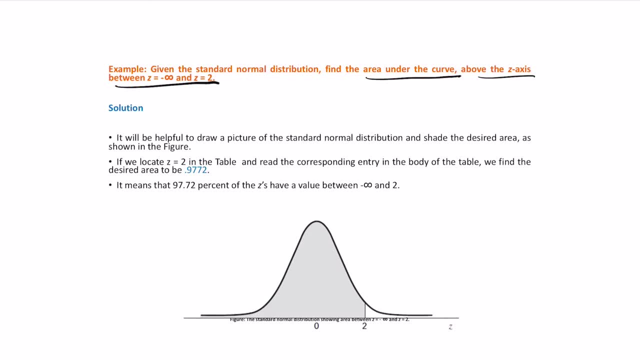 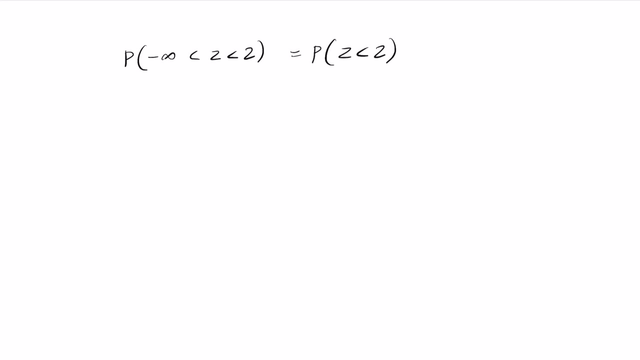 equal to negative infinity and Z equal to 2.. Now let's try this problem. So they're asking you between minus infinity and 2.. So it basically means they are asking you to find Z less than 2. Nothing else. They are not asking you anything else. How would you find it from the table? So let me find the table first. 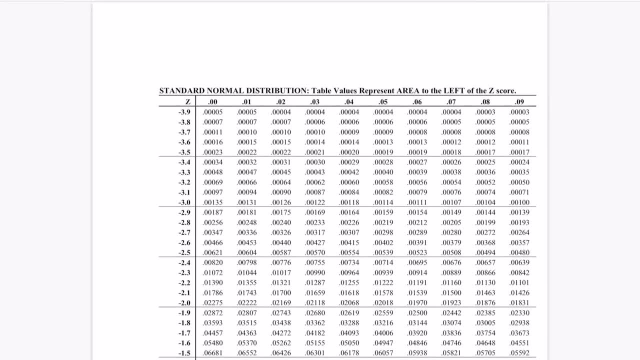 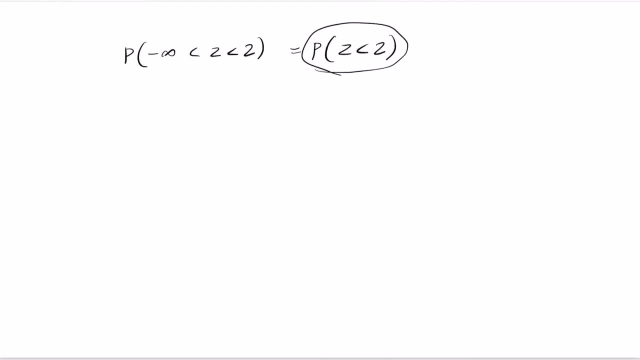 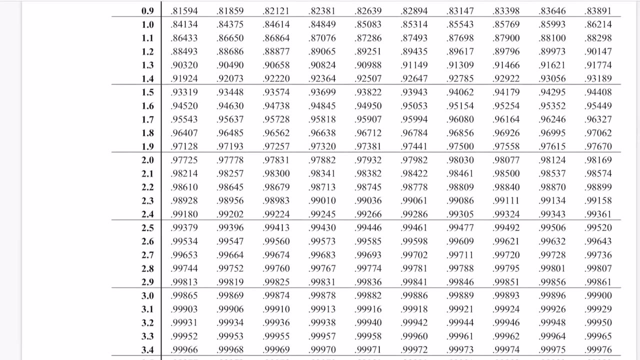 So what you see here is an example of a standard normal distribution table. Now we have to find the value for Z less than 2.. So in the normal distribution table we have to find the value for 2.. So this is the value. So notice that. 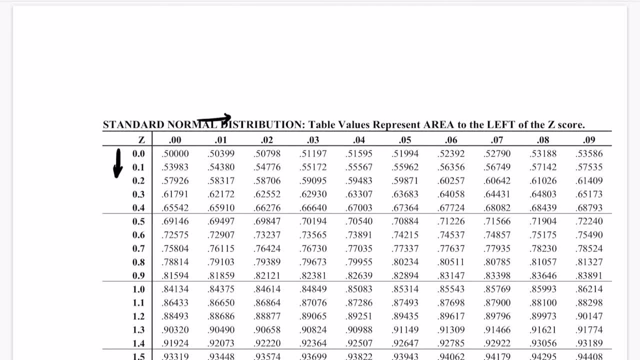 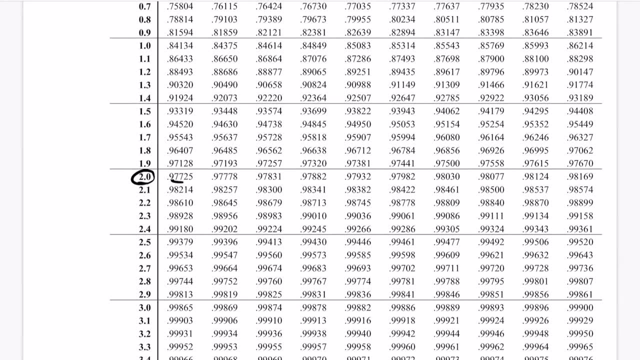 Notice the Z column here and notice the second decimal column here We have to find for 2.. So this is the value 2.. And I'm going to find it for 0.00.. So 2.00.. So this is the value. 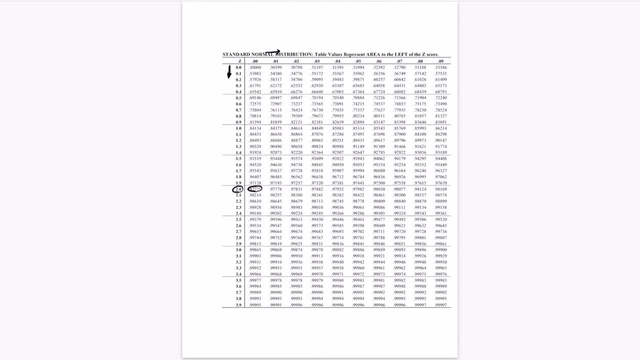 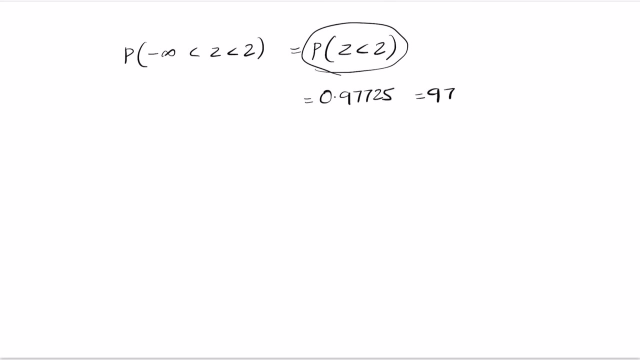 Now 0.97725.. So when you write it down, so this is the answer 0.97725.. Or you can write it as 97.725 percent. So this is the probability of value Z less than 2.. 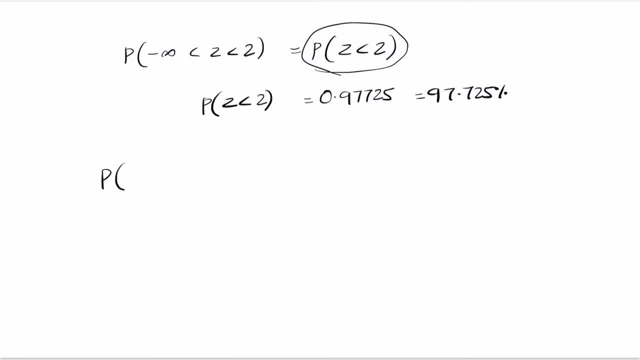 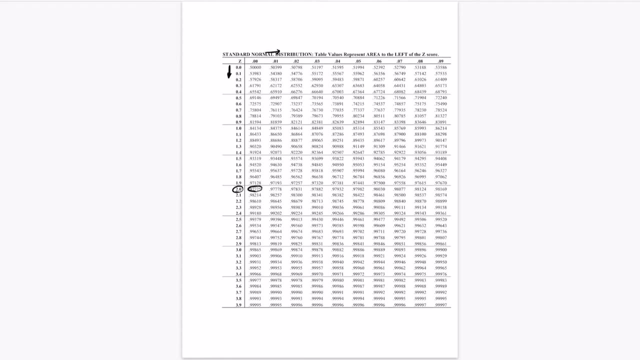 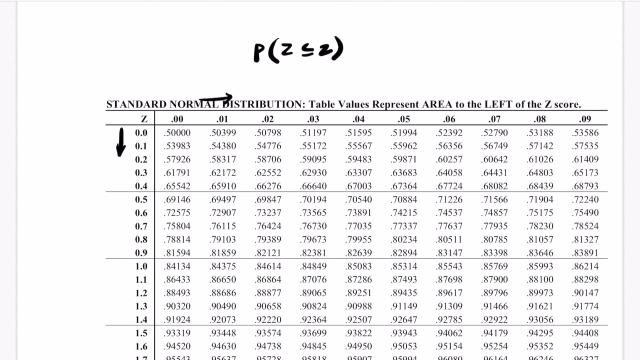 Now, in the same way, Try to find- let's try to find- Z greater than 2.. How would you find that greater than 2?? Notice that in the probability table all the values are written in such a way that the probability that you find is Z, less than or equal to Z. 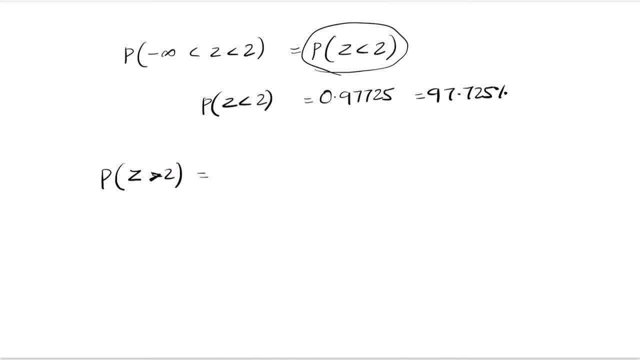 So which means that if you take Z less, so what we are doing here is that if you take this distribution here, when we take the value for 2, so when you take z equal to 2, so we are finding this entire probability here. so the table basically. 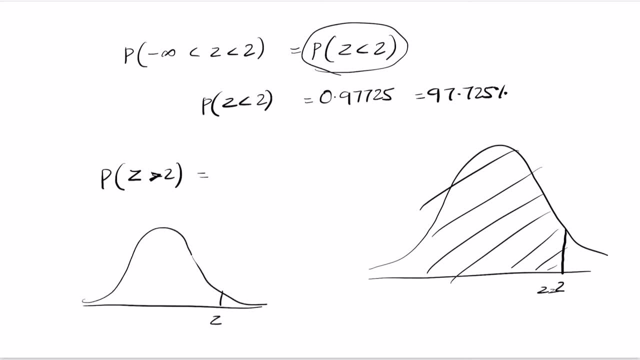 considers that if you take any z value, so if this is the z value, what is the value that you are finding? is this entire probability, this entire area? now, if i want to find z greater than 2, so then you are finding this area here, this part here. how would you find that here so that you would 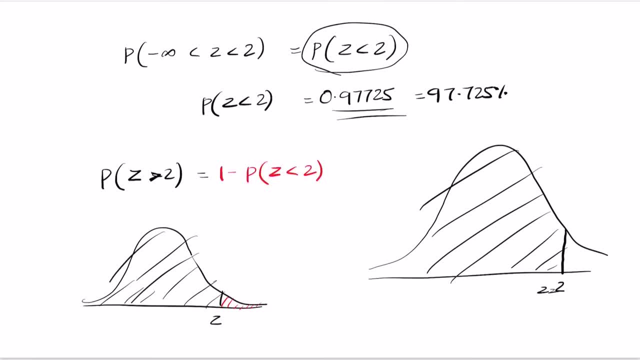 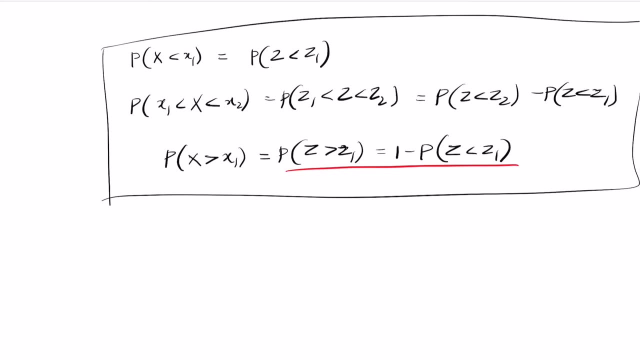 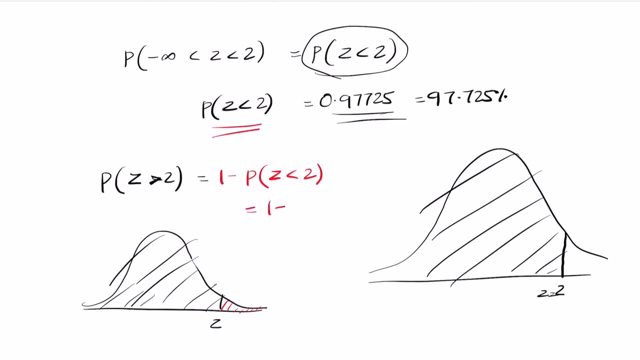 write it as 1 minus p of z less than 2. remember the formulas i told you about. so the formulas that you that i told you about. so use the formula here. when you write greater than, write it as 1 minus p of z less than so how would you find it here? 1 minus z less than 2, the value is 0.97725. 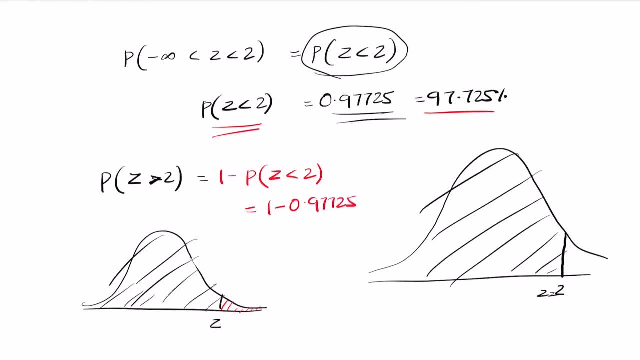 so 0.97725. so use a calculator. so the value is 1 minus 0.97725, 0.97725, so that value becomes 0.02275 or 2.275 percent. so this is the value of p, of z greater. 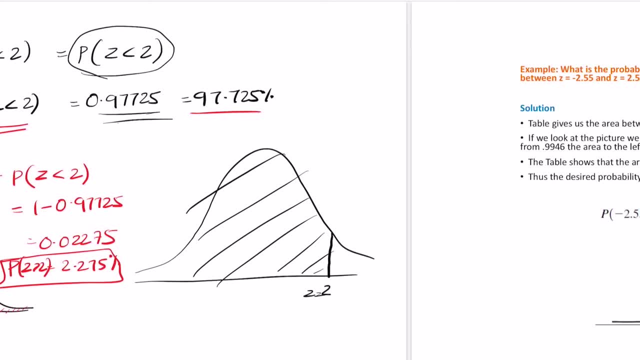 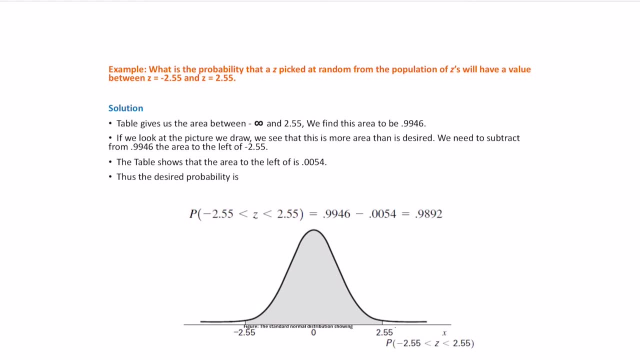 than 2.. now, in the same case, let's say: if i want to find something else, let's say i have. they're asking you to find the probability between z less than z equal to minus 2.55 and z equal to 2.55. so 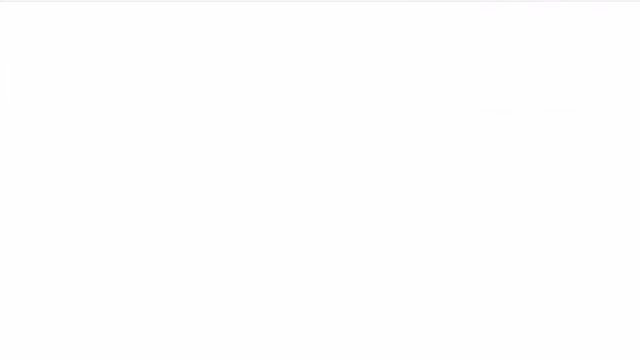 how would you find the probability between z less than z equal to minus 2.55 and z equal to 2.55? so how would you find it in the table now? so first thing first always draw the diagram so that it becomes easier to understand the topic. so this is the distribution. let's consider that this value is minus 2.55. 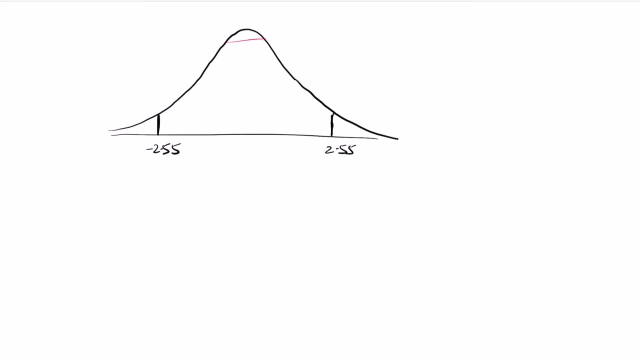 and this is 2.55. so they are asking us to find the area of this. this area, how would you find it from the table? so the you can write it as p of minus 2.55, less than z less than 2.55. so how will you find this from the table? remember the formula. so p of z1 less than z less. 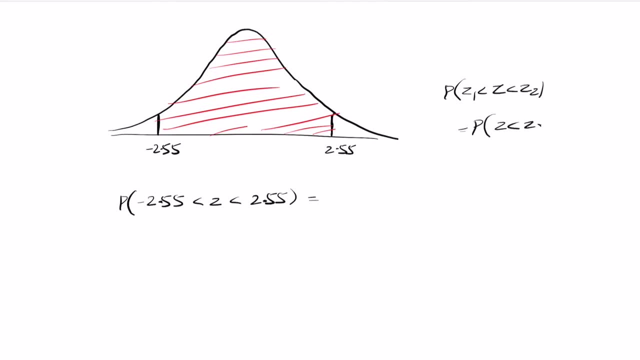 than z2 can be written as p of z less than z2 minus p of z less than z1. so p of here z less than 2.55 minus p of z less than minus 2.55, 2.55. so first things first, we want to find 2.55. what is the value? so the first value is 2.5. 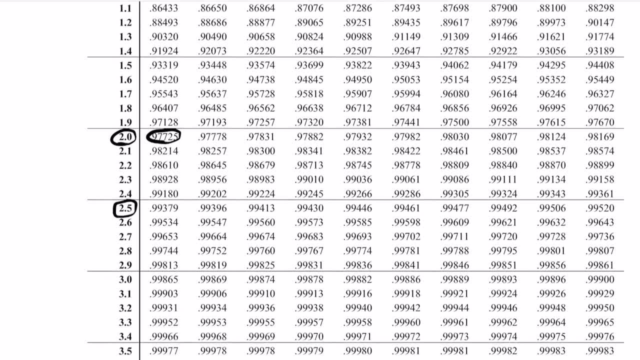 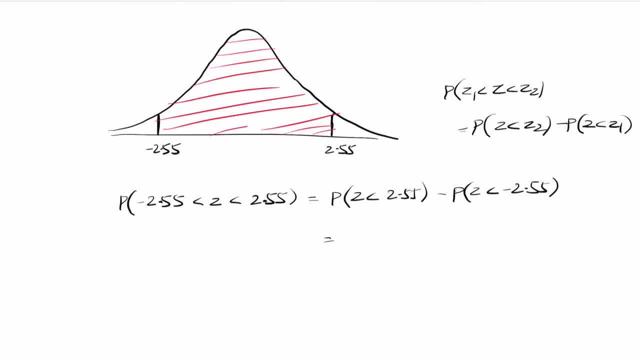 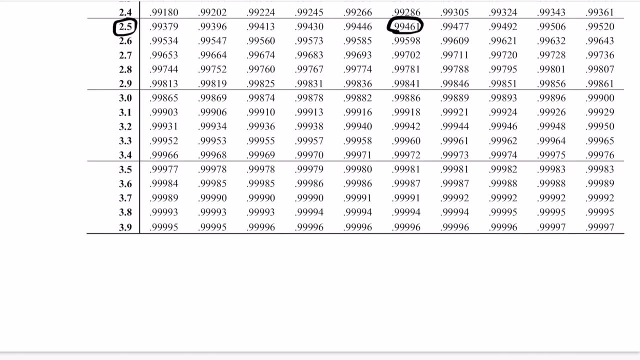 and 2.55 is this row, so that row is going to be 0.99461, so write down the value so that is 0.99461. this is the value for z less than 2.55. now we want to find z equals minus 2.55. 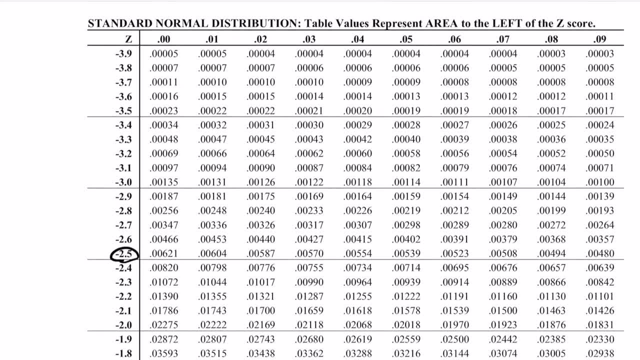 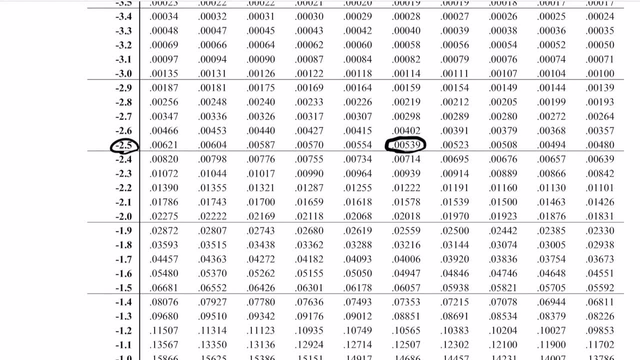 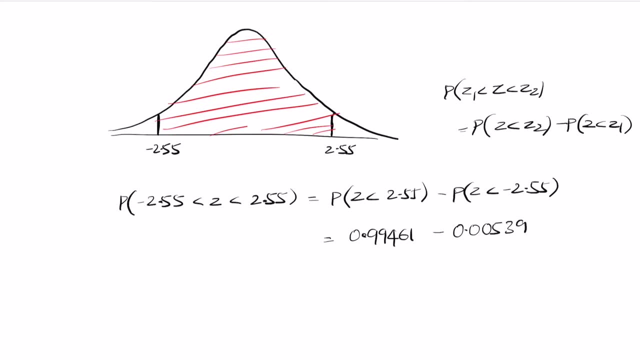 so we have minus 2.5 and we have to find 0.05 under this again. so this is 0.05. so under that you have 0.00539 minus 0.00539. now subtract the two values, you have 0.99461. 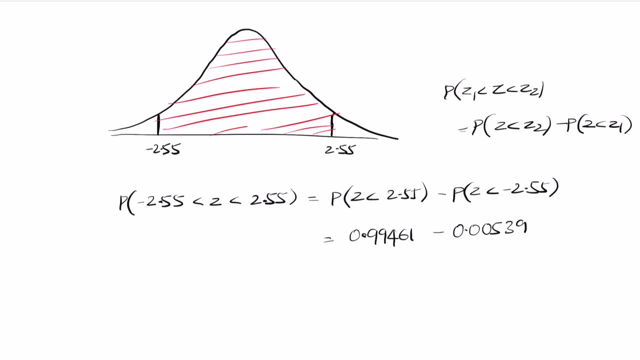 minus 0.0053, 9, so that gives you a value of 0.98922, or we can write it as 98.922 percent. so this is the probability between minus 2.55, less than z, less than 2.55. now, in the same problem, try to find p of. 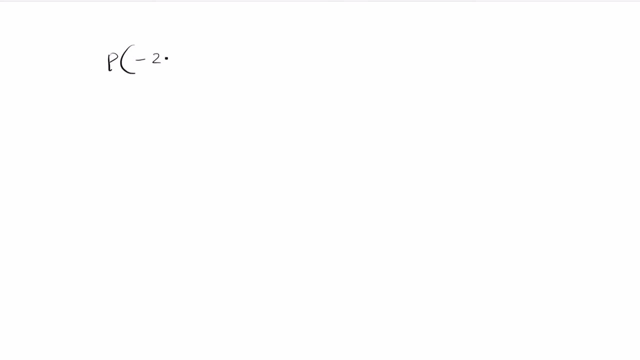 minus 2.55, 46 less than z less than 2.46. so i'm going to attach the table with the problem. so in the canvas. so make sure you download the table first and keep it on your computer so that when practicing it becomes easier. so try this problem now and if that is done, try z less than 3.21. 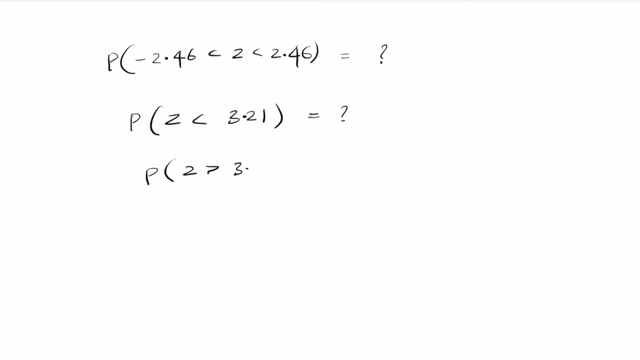 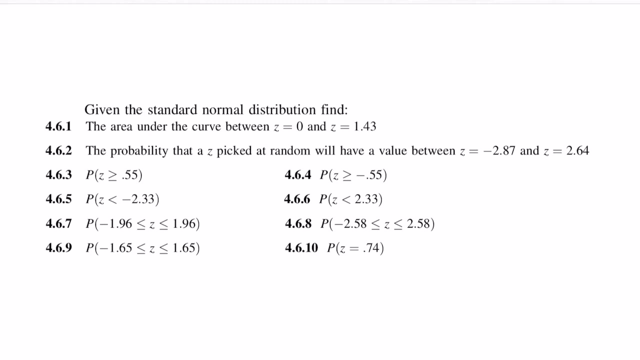 and also find z greater than 3.01. so pause the video right here and try to solve these problems. so if you are done with the last example, so pause the video right here and try to solve these problems. so let's recap how to find the z values. so when you have p of z less than a or p of z, 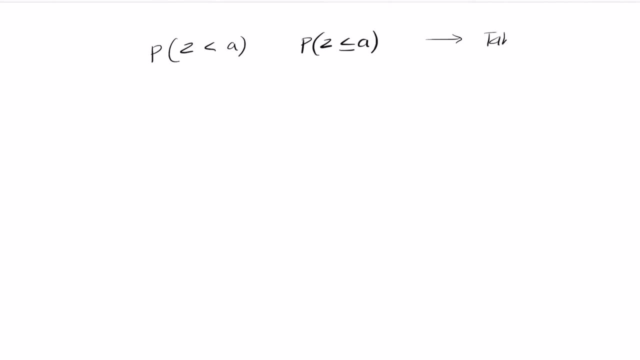 less than or equal to a. so just find the table and for the z value find probability. all right, so that's it directly. but if you have z greater than a or p of z, so let me write it as b here, so that it becomes separate. so, or z greater than equal to b, how will you write? 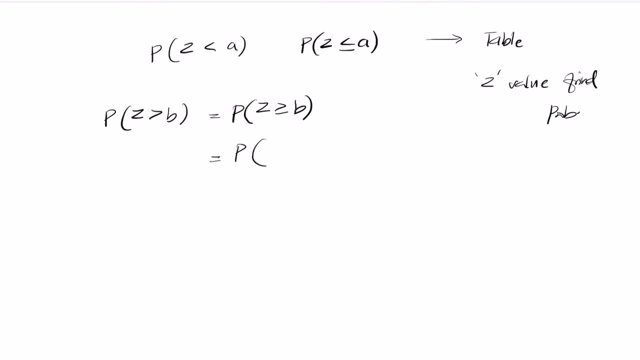 this formula. both of them are the same. so the formula is 1 minus p of z less than b, right? so find now the probability for b and calculate probability and substitute it into this value and finally find the answer. If you have two values- a less than z less than b, then the formula is p of z. 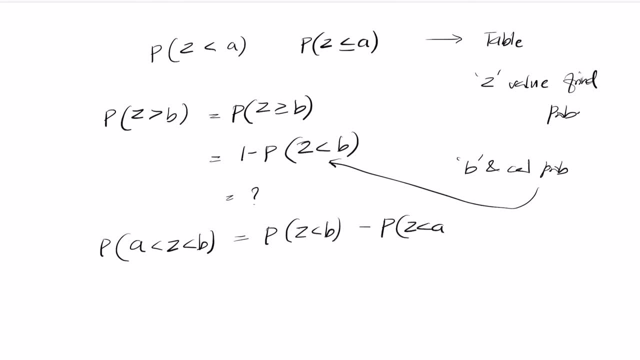 less than b minus p of z less than a. So find the probability for b and find the probability for a and finally find your answer. So these are the two main formulas to remember. So this is one formula and this is the other formula. So remember these two formulas, it makes it easier to understand the 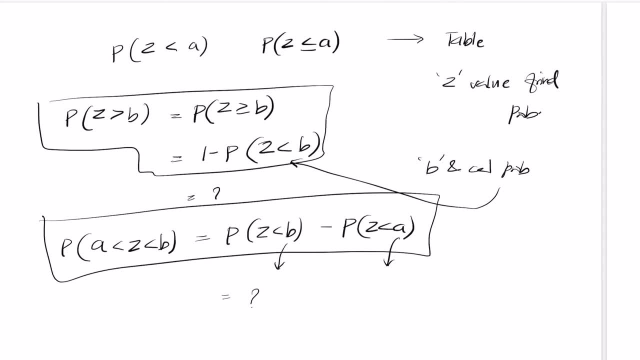 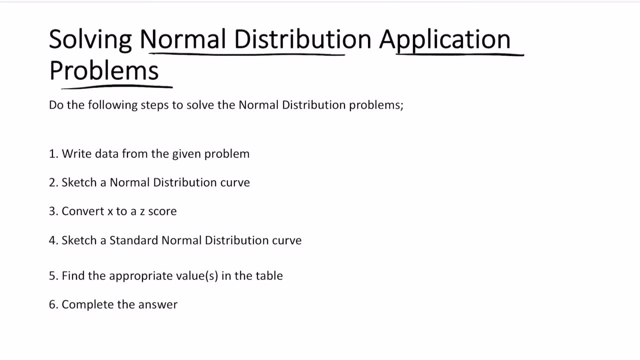 problem. Now let us come to a normal distribution application problems. How do you apply normal distribution to the problems? So we use the following steps to solve normal distribution problems. First, write down the data that you have in the problem. Second, sketch a normal distribution. 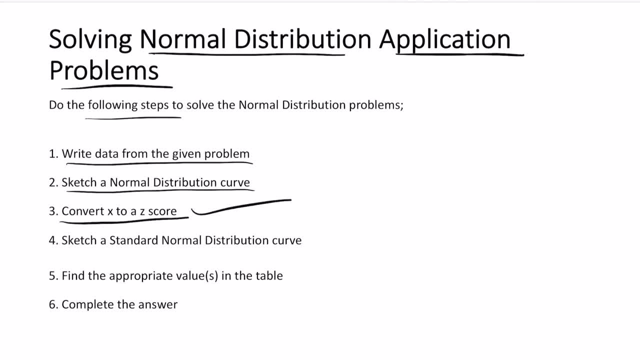 curve and then write down the data that you have in the problem. So this is the normal distribution curve. And third, convert x to a z score using the formula x equal to sorry, z equal to x minus mu by sigma. And fourth, sketch the standard distribution curve. and finally, five, find the values from the 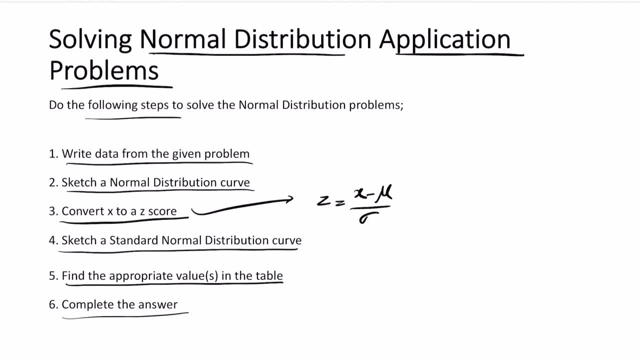 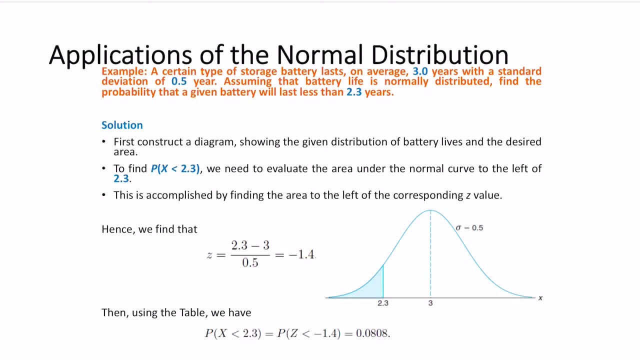 table and six complete the answer. So these are the steps that are required while solving the problem. Now let us take a problem and let us see if we can solve this problem. So a certain storage battery. So let me write it down separately. So now let us try and solve this problem. So first thing we want: 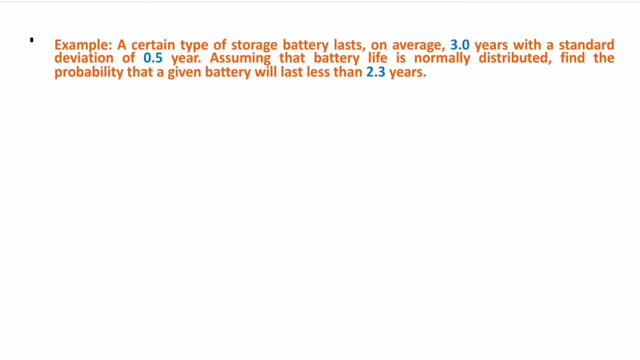 to do is note down the data. So in the problem it is given that a certain type of storage battery lasts, on an average, three years, with a standard deviation of 0.5 year, Assuming that the battery life is normally distributed. given that the battery will have less than 2.3 years, find the 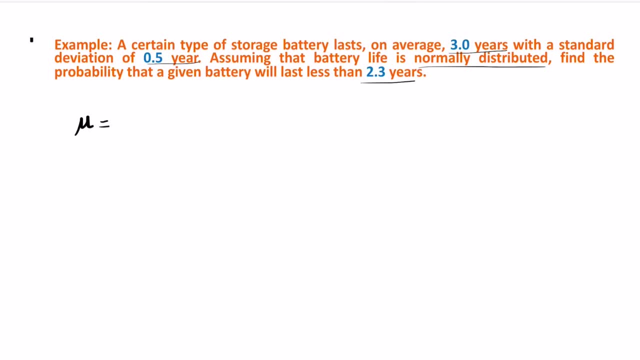 probability. So the first thing is mu, So the value for mu is given as three years. So note down three years And the standard deviation sigma is 0.5 years. And they are asking you for the probability that the battery will last less than 2.3 years. So the probability of x less than. 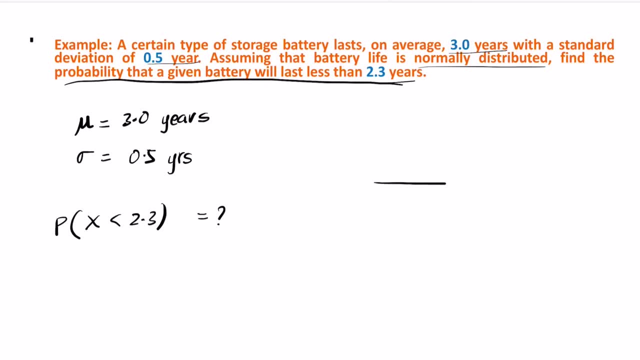 2.3.. So this is the probability that they are asking for. So if you draw the normal curve now, you notice that this is the mu value, which is 3.0.. And the standard deviation here, sigma, is 0.5, and they are asking you to find the probability of 2.3. so, for example, let us consider that this: 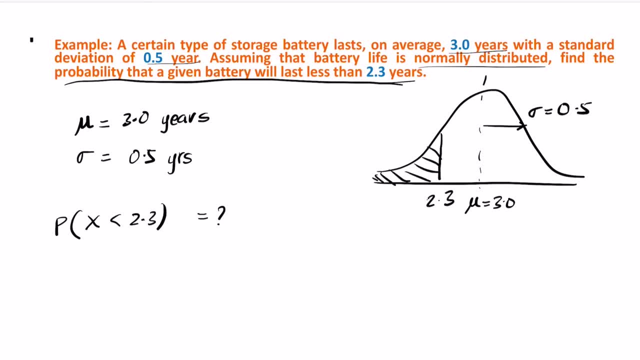 is somewhere 2.3. so they are asking you to find this area. so to find this first we need to convert it into the z score. so the z score formula is, as z, equal to x minus mu by sigma, so x is 2.3. 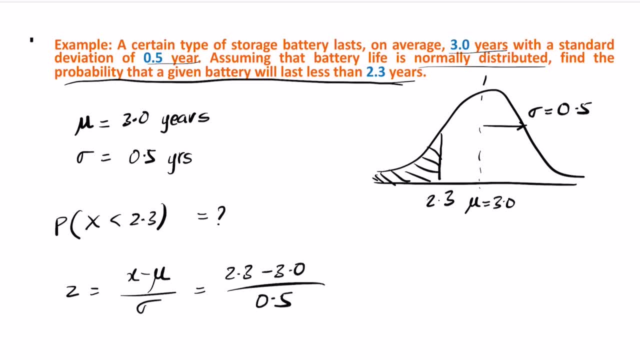 minus 3.0 by sigma is 0.5, so that becomes minus 0.7, by 0.5, so that becomes minus 0.14. so this is the value for the problem. so you can check it. so 0.7 over 0.4. 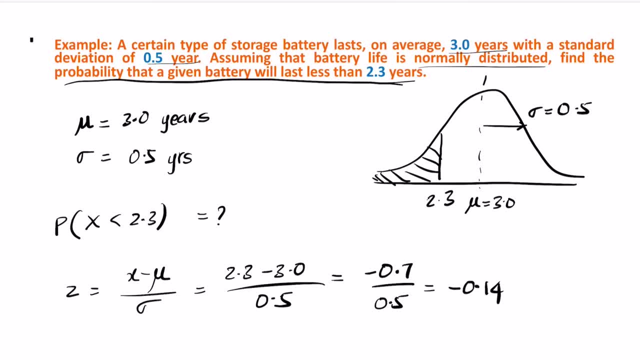 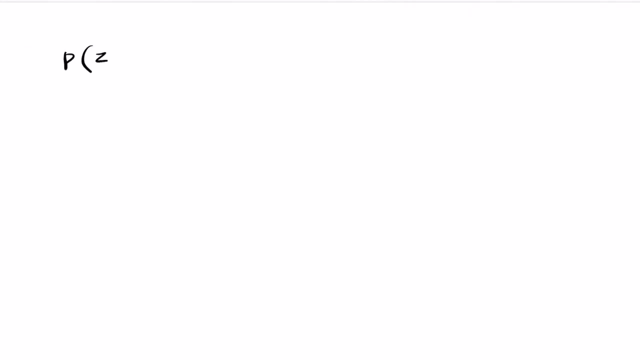 0.5 is 1.4- i'm sorry- minus 1.4. so this is the value of z. so now we can convert this p of x less than 2.3 into p of z less than minus 1.4. now we are finding the probability of z less than minus. 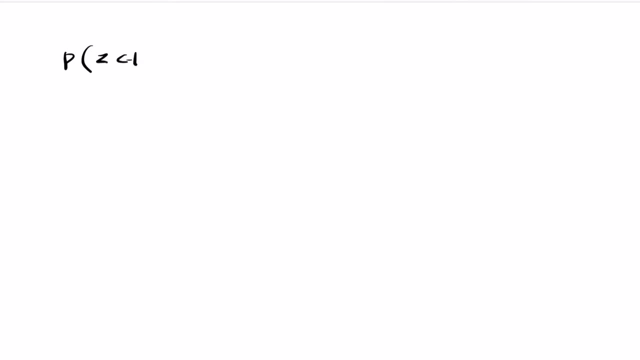 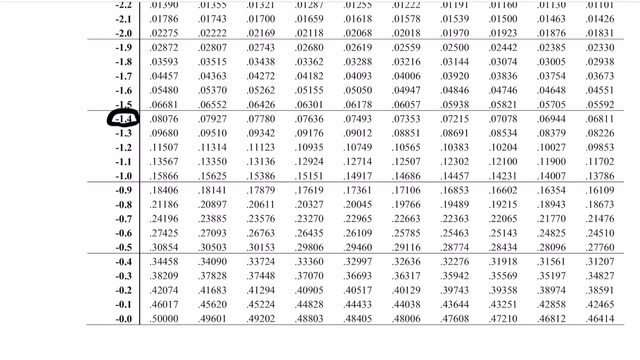 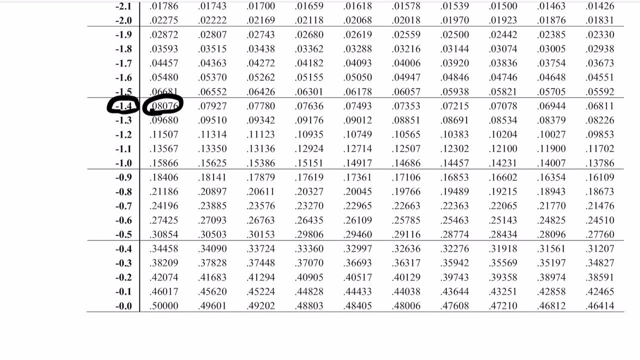 minus 1.4. how will you find this? so let's go to the table back again: minus 1.4, so this is minus 1.4 and 0.00, so minus 1.40 total. so this is the value 0.08076. 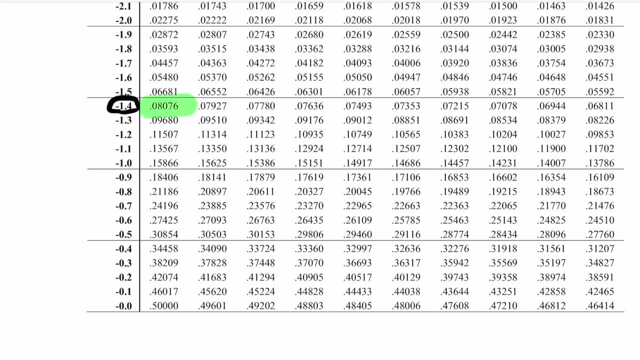 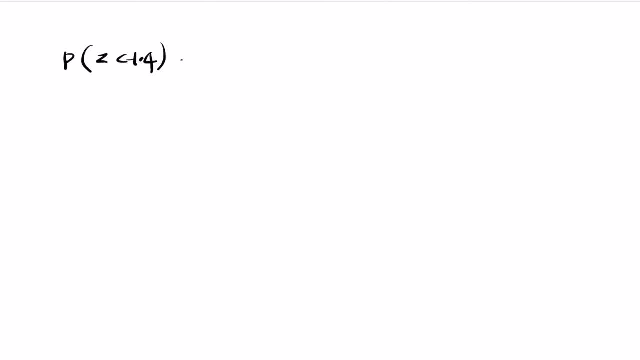 right. so this is the value: 0.08076, now 0.08076, so in percentage, if you want to write it, divide this by 100, so you get 8 point 0.076 percent. so, which means that the probability of x less than 2.3 years is 8.076 percent or 0.0876. 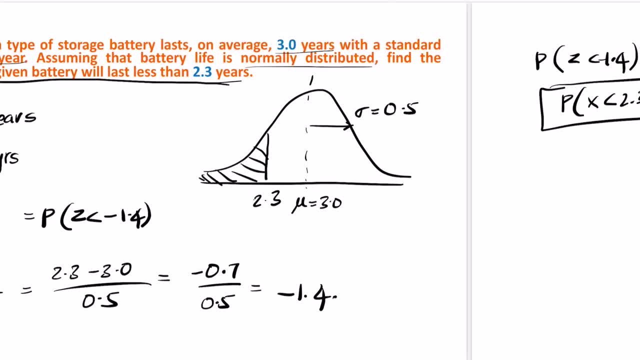 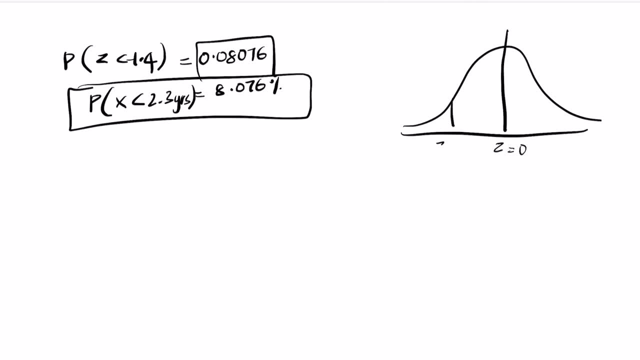 so this is how you can convert the problem from one value to the other value. so if you draw it in terms of the standard normal distribution, so this is the z value equal to 0. this is the z value that you have: 1.4, sorry, minus 1.4. 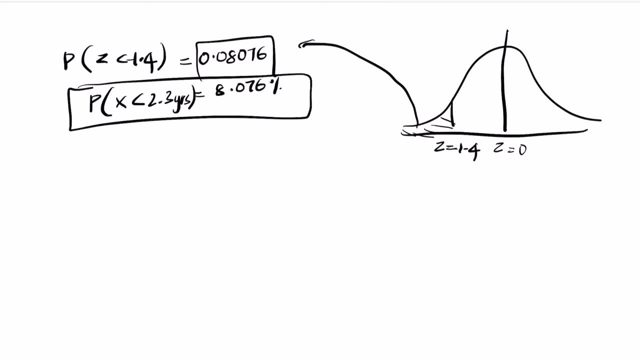 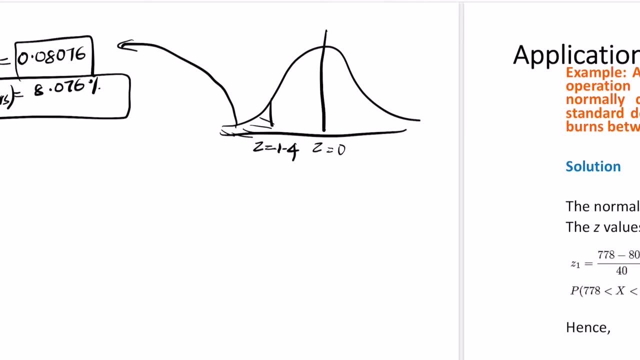 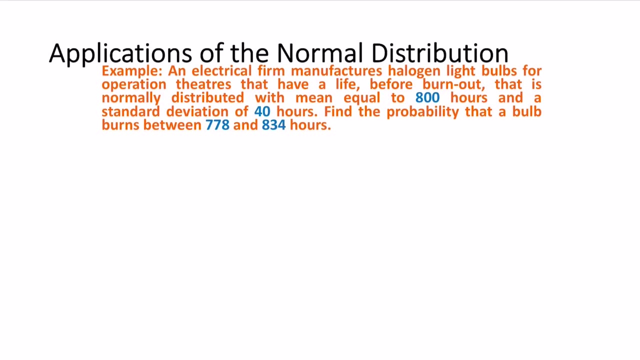 and this is the area that you found as this problem. so this is how we can convert an applying normal distribution into the general problem. see, let's try another problem now. let's try this problem here. what is the given here? so 800, so 800 is. 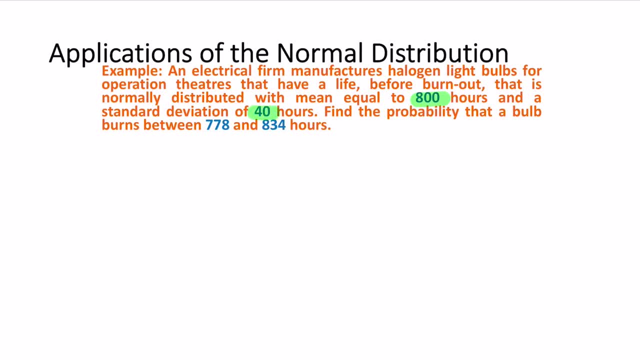 the value of mu, standard deviation is 40. they are asking you to find between 778 and 834. down the data first: mu is 800, sigma is 40 and they are asking for probability of 778 less than x, less than 834. so which can be written as the probability of x less than 834. so the first. 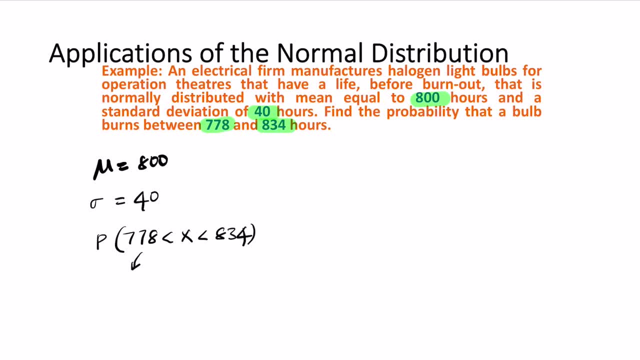 things first. let's try to convert. so you have two z values. so this is x1 and this is x2. so first find z1. so z1 is x1 minus mu by sigma. x1 is 778 minus 800 by 40.. z2 is x2 minus mu by sigma. 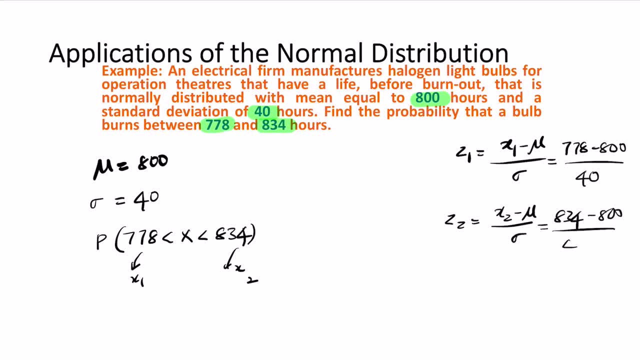 so which is going to be 834 minus 800 by 40.. so 778 minus 800 will give you 22 by 14 for z1 and z2 is 34 by 40. sorry, this is negative 22 by 40.. 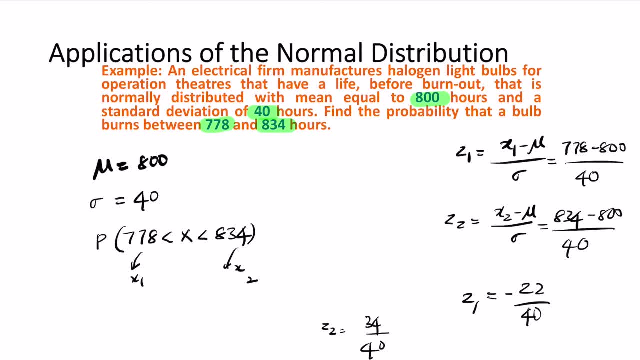 so when you calculate 22 by 40, so the value is minus 0.55. so for 34 by 40, so that value is 0.85. so now write it down in terms of z. so the probability of z1 less than z less than z. 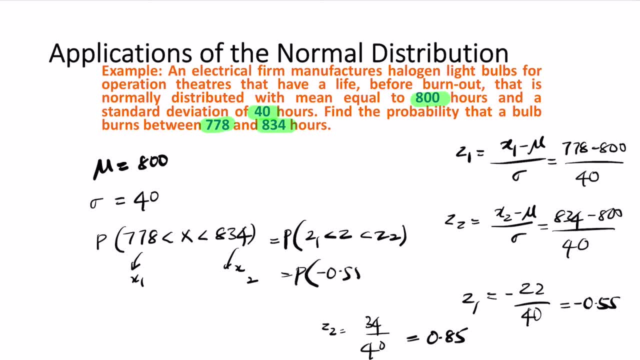 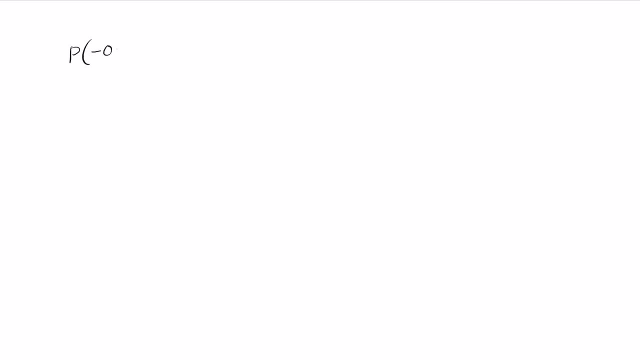 so the probability of z1 is minus 0.55, less than z less than 0.85. so this is the probability that you are finding. so now let's note this down on a separate page. so probability of minus 0.55 less than z less than 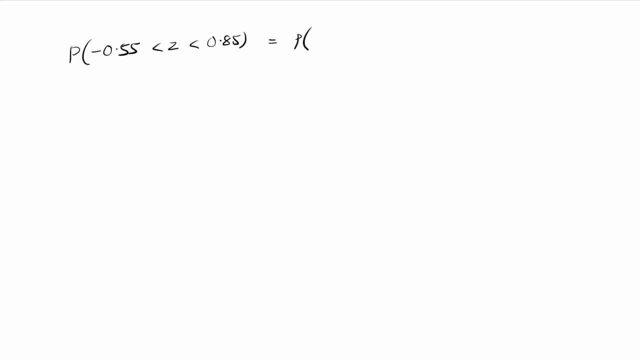 0.85. so this can be written as probability of remember a less than z less than b. so z less than b first. so z less than 0.85 minus the probability of z less than minus 0.55. so probability of z less than 0.85 again go back to the table. 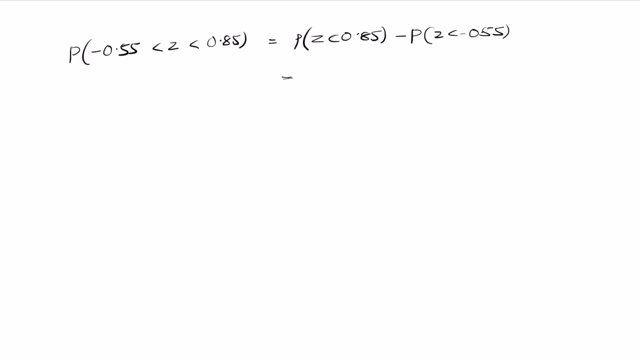 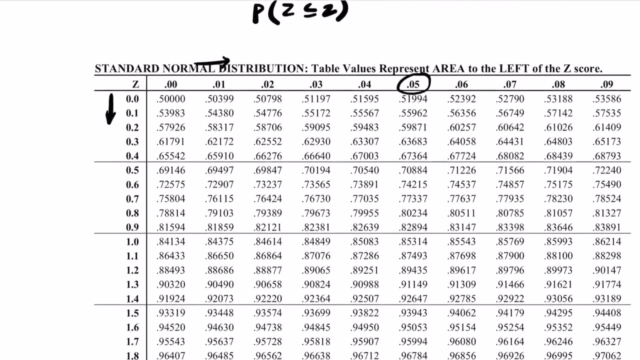 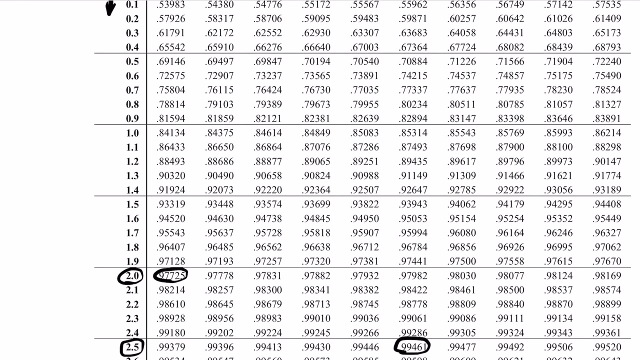 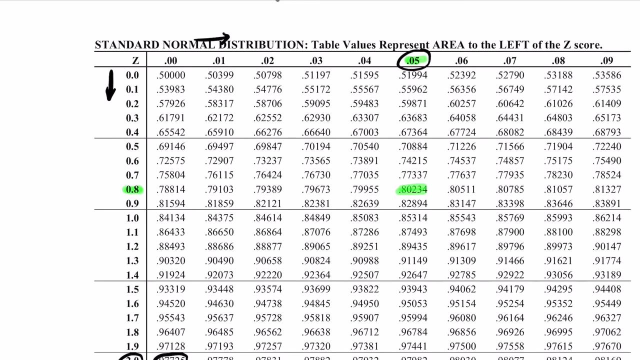 so we are finding for minus 0 z 0.85 first. so this is 0.85 first. so you have 0.8 here. So you have 0.8. here We are finding 0.85.. So this is 0.5.. So 0.85 becomes 0.80234.. 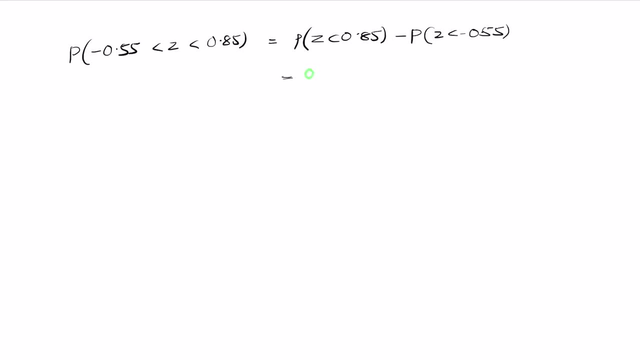 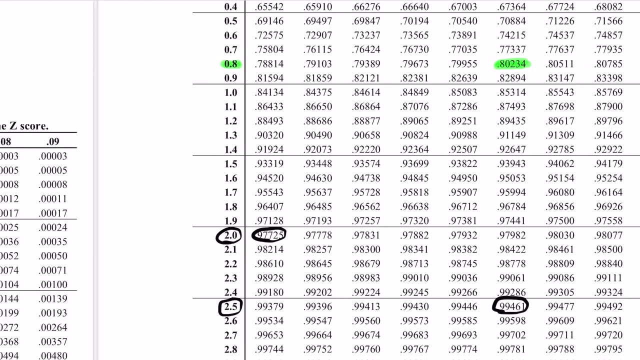 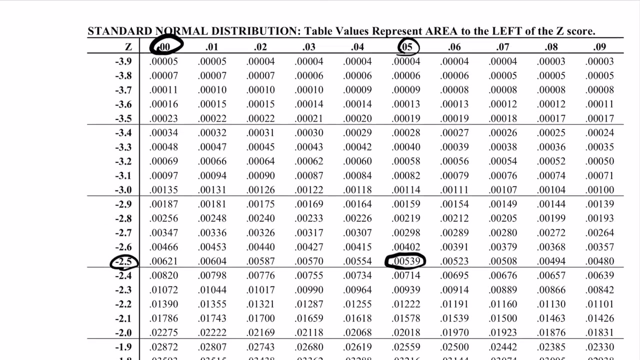 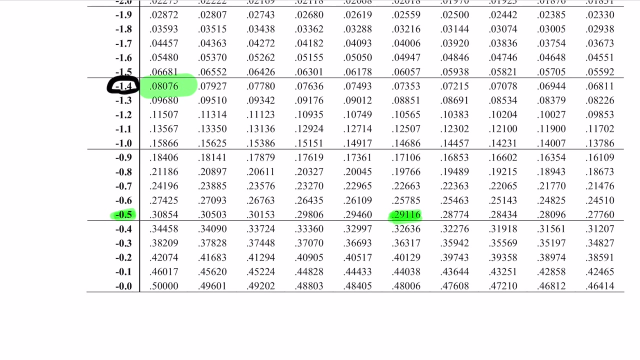 So write it down: 0.80234 minus minus 0.55.. So minus 0.5, and 55 is here, So in this one. so this is the value Minus 0.29118.. Correct: 29116.. 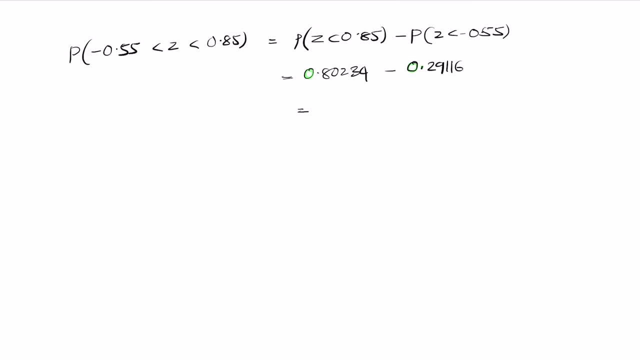 So 0.29116.. So 0.80234 minus 0.29116.. That gets you a value of 0.51118.. So this is the probability of minus 0.55. less than that, less than 0.85.. But this is not the 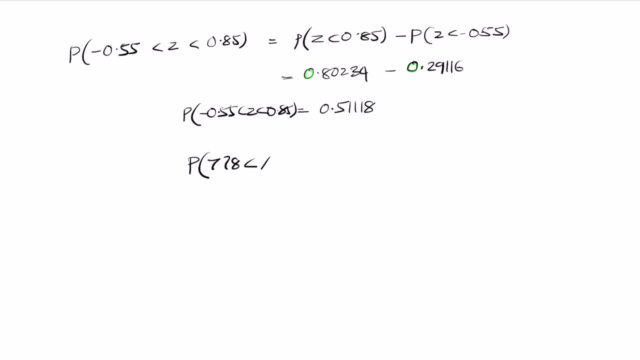 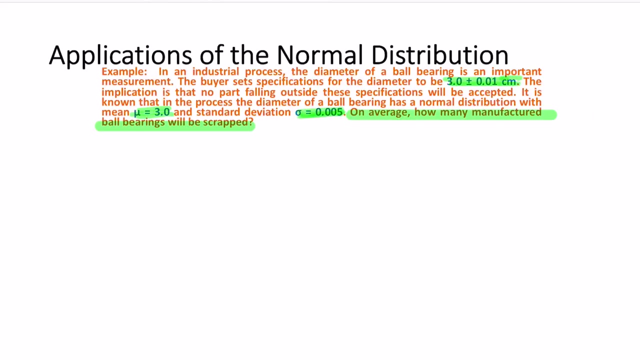 original probability. The probability originally is 778, less than x, less than 834.. This value is 0.51118 or 51.118 percent. So this is how you can find the probability: by applying conditions. So what is the data given? You have mu, which is 3.0, and sigma, which is 0.005.. 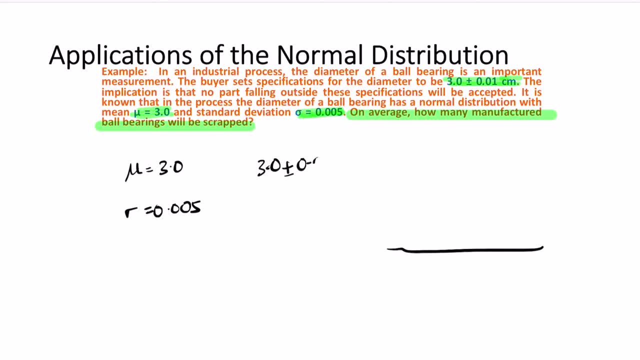 Now the bearing diameters. The bearing diameters that are given is 3.0 plus or minus 0.01 centimeters. So if you take the distribution table, if this is 3, so these are the two values. So 3 point. 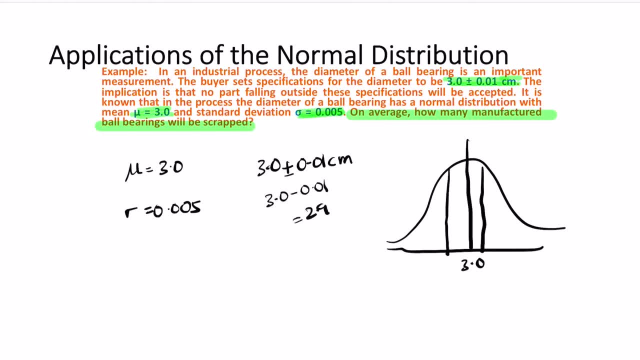 if you write it as 3.0 minus 0.01,, that gives you 2.99.. And 3.0 plus 0.01, that gives you 3.01 centimeters. So this is 2.99 and 3.01.. So this part is accepted, So which is rejected. 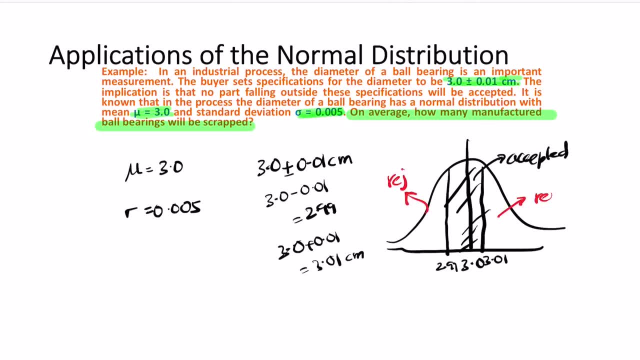 Rejected here. So these are the parts that are rejected. So this part is rejected and this part is rejected. So let me write down the probabilities that way. So we are finding two probabilities. One value is probability of z less than 2.99, which represents this area, And sorry, 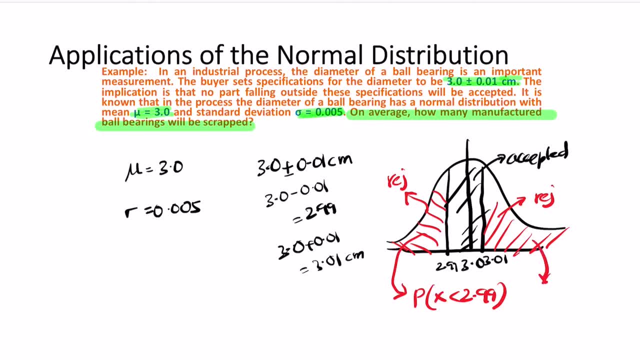 probability of x less than 2.99.. And this part, which is probability of z- sorry, x- greater than 3.01.. Probabilities that we have to find: x less than 2.99 plus probability of x greater than 3.01.. 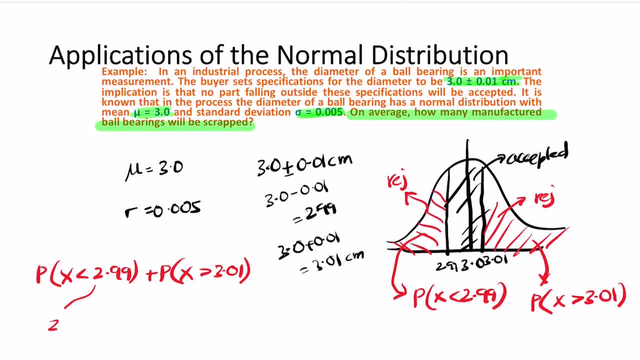 So first things first, convert these into z values. So what will be the z value for this? So z becomes x minus mu, by sigma, which is 2.99. minus mu is 3.0, by sigma is 0.005.. So you have 2.99 minus 3. 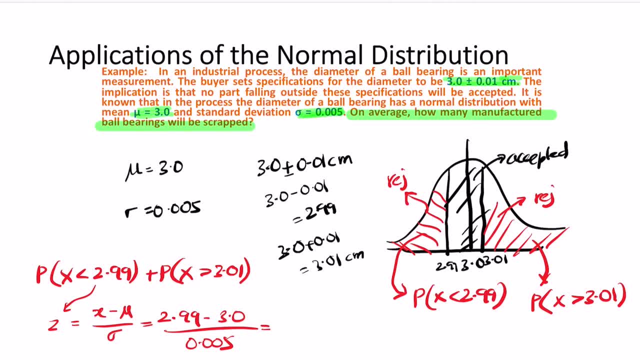 over 0.005.. So that gives you a value of negative 2.. Now for the second value, for 3.01.. So when you find it, you get 3.01 minus 3.0 by 0.005. So that is 0.01 point by 0.005. So that is 0.005.. So that is 0.01. 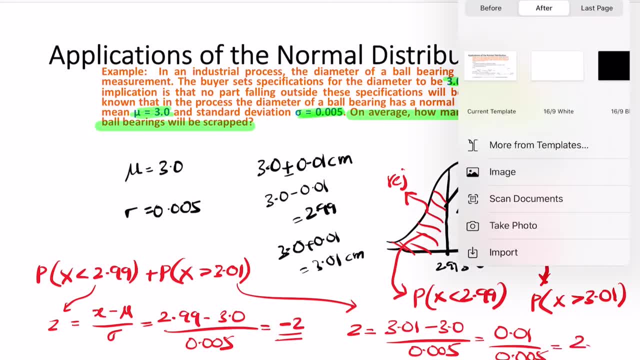 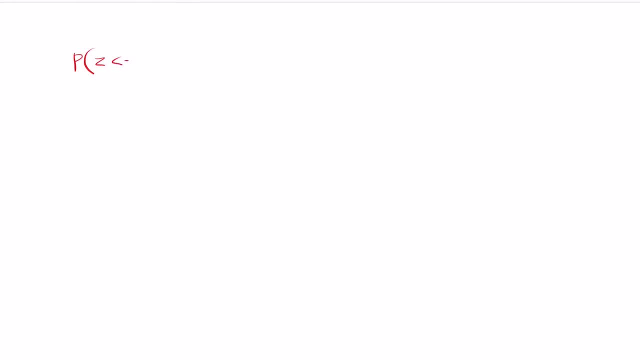 phi that becomes 2. so when you write it down as the probabilities, so the probability of x less than 2.99 becomes z less than negative 2 plus the probability of z greater than 2. so we know the probability of z greater than minus 2 that you can calculate directly from. 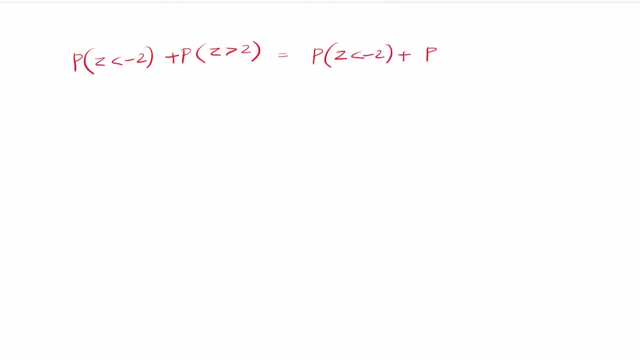 the table. but z greater than 2 becomes 1 minus p of z less than 2.. Now, how would you find this? so, because this value in general, if you actually find out the value, you will notice that this value actually becomes nearly equal to 1, so, which is something that we do not want to do. so what? 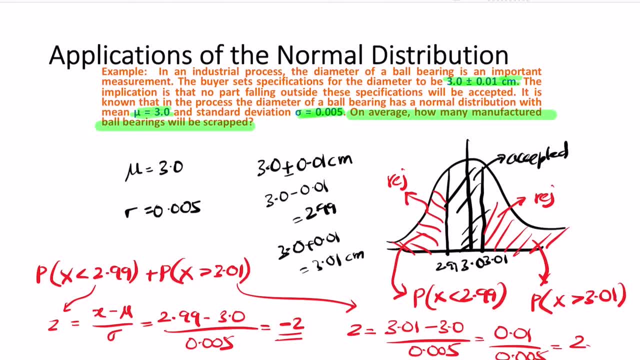 we are going to do is we are going to write down the probability of z greater than 2, and we can do now, rather than doing this, is notice that these are the two values, so this part is accepted, so which means that anything other than that is rejected. so, for this value, what we can do, 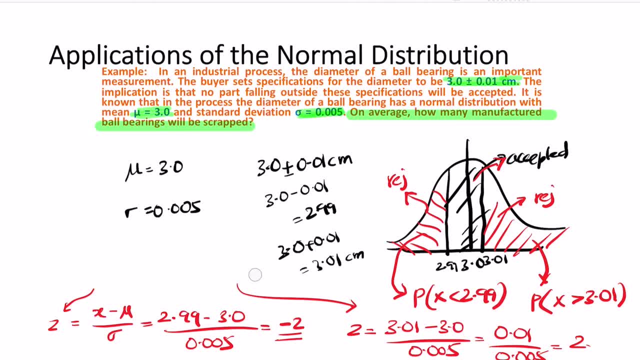 now is we are finding the exact same z values. we have found the exact same z values, but rather than finding it this way, let us find p of 2.99, less than x, less than 3.01. so this value for this z value is minus 2. again, for that z value, it is 2.. 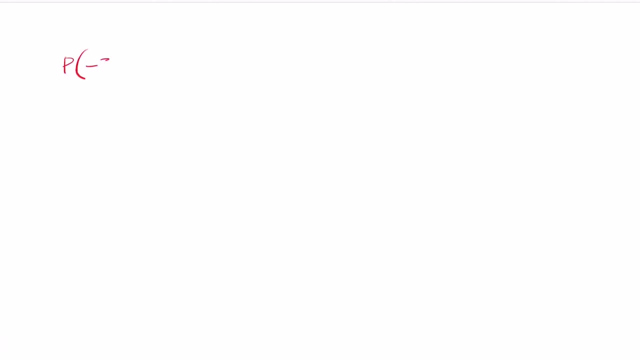 So that probability is p of z minus 2, less than less than z less than 2.. So if you already remember, from the table you can find the formula directly as p of z less than 2 minus p of z less than minus 2.. So from the table, what is the value for 2? so the value for 2 is 0.97725, 0.97725, minus for minus. 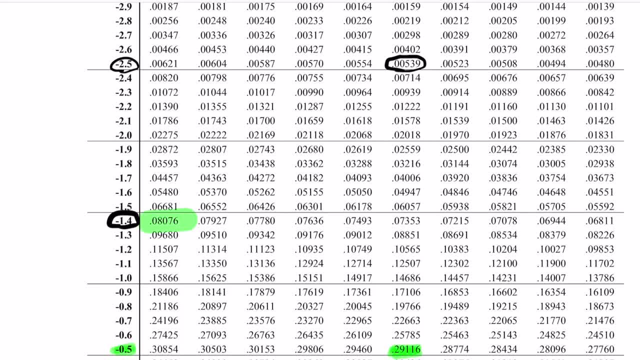 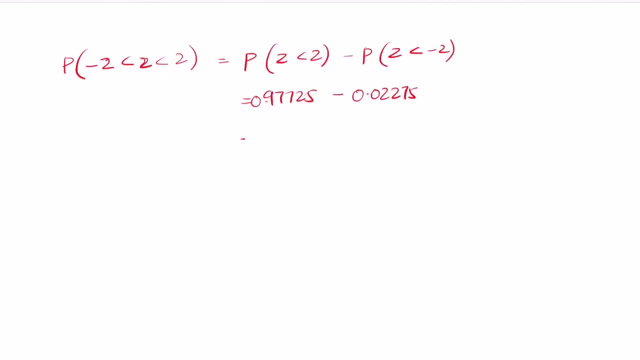 2. so for minus 2, the value is 0.02275- 0.02275. so that value is going to be. so let us find out the value: 0.97725 minus 0.02275, so that gives you 0.9545.. 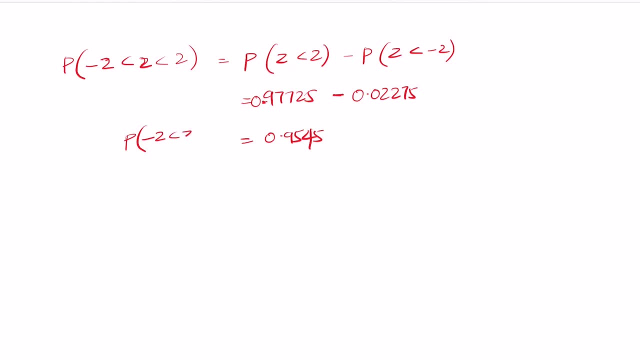 So this is the probability of minus 2 less than z less than 2.. So this part is the accepted part. what is the rejected part then? so rejected is 1 minus accepted. so 1 minus 0.9545 becomes 0.045.. 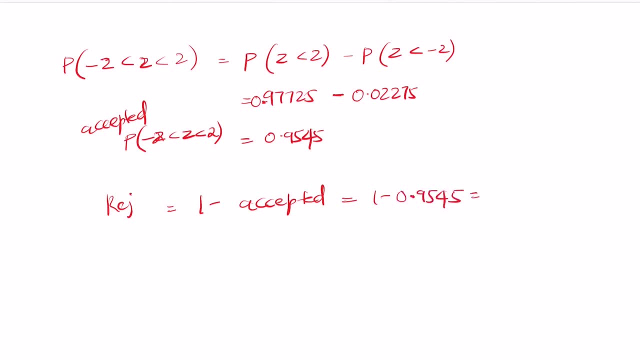 So this is the probability of minus 2, less than z, less than 2.. So this part is the accepted part, 1 minus 0.9545, or we can write it as 4.55%. So this is the amount that will be end up. that will. 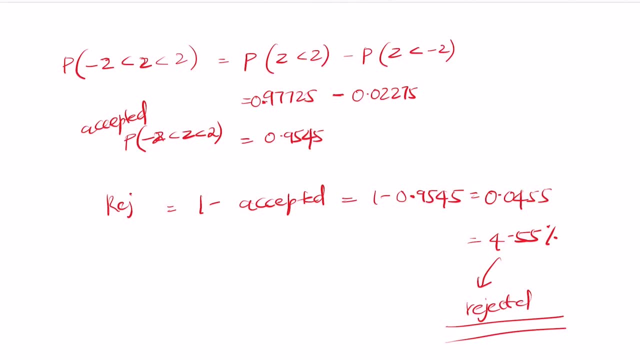 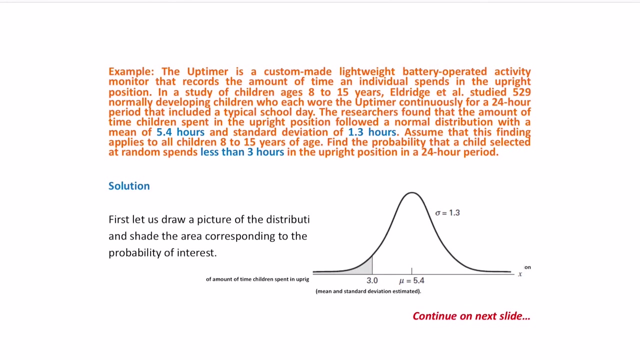 end up being being rejected. So this is one another way for finding the same answer, but using one another method, but the answer is still the same. so you are finding the exact answers being the same. So this is how you can apply problems for normal distribution. Now pause the. 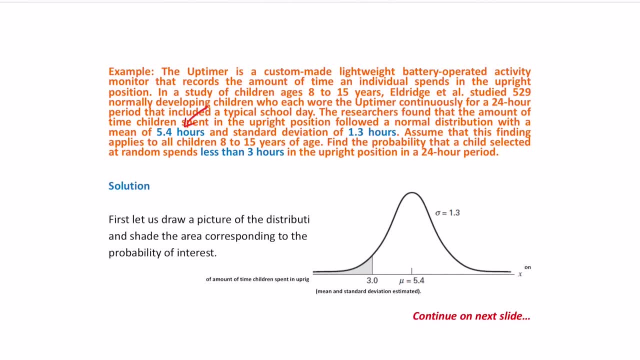 video right here and try to find this problem. So here this is the value of mean and this is the deviation, and they are asking you for less than 3.5.. So p of x less than 3.. So try to convert it into z value and then find the probability. So pause the video right here and try to solve.